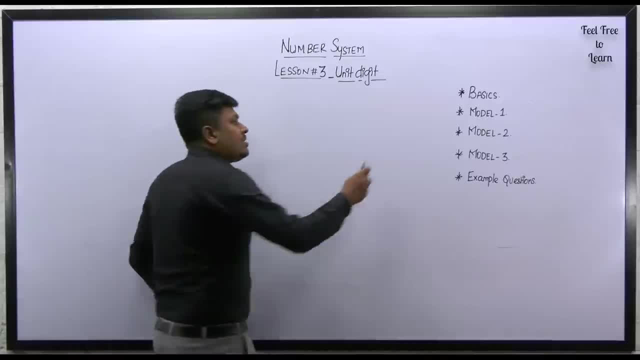 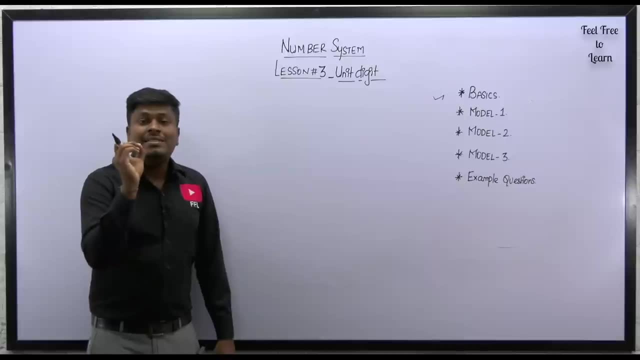 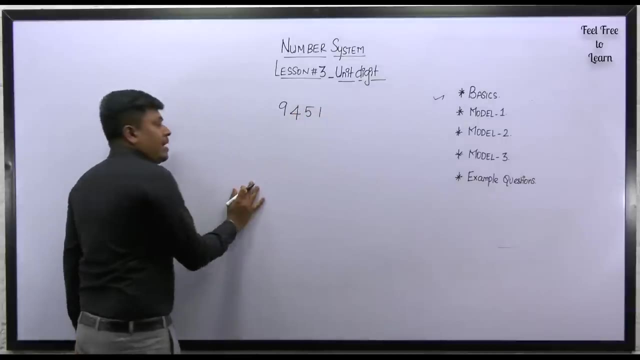 So before that, first let me learn the basics, right? So what is called as an unit digit? So listen here. unit digit is, whatever the number be the last digit of the given number. For example, let me take any number, 4951, right 9441.. If they ask: what is the unit digit of this? 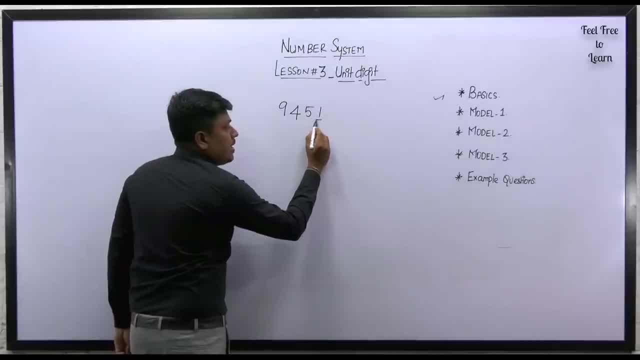 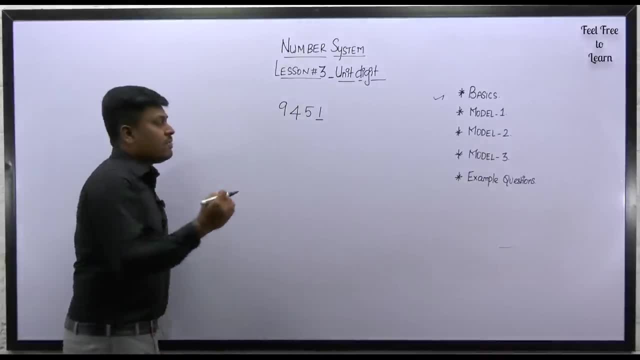 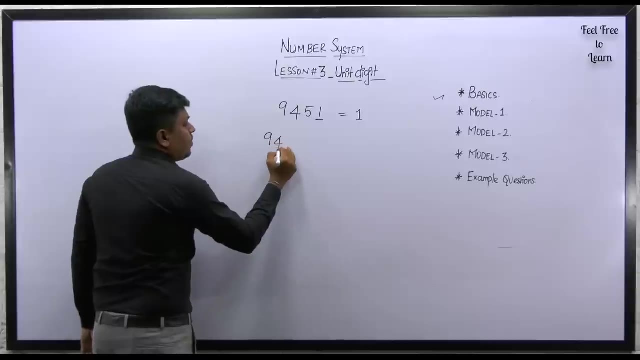 number is the last digit, understood. The last digit of the given number is called as an unit digit, understood or not. So, finally, the unit digit of the given number is 1, understood or not? any number it let me take 946345.. So in case, if they're asking what is the unit digit of the given, 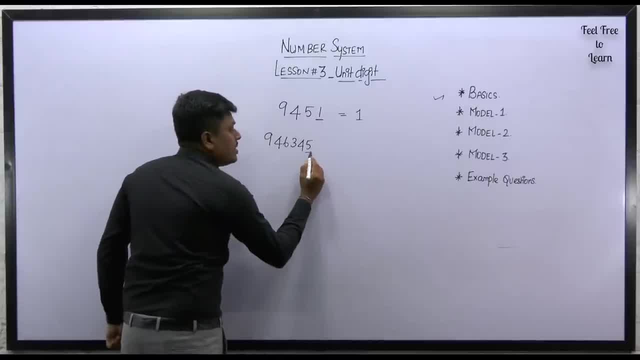 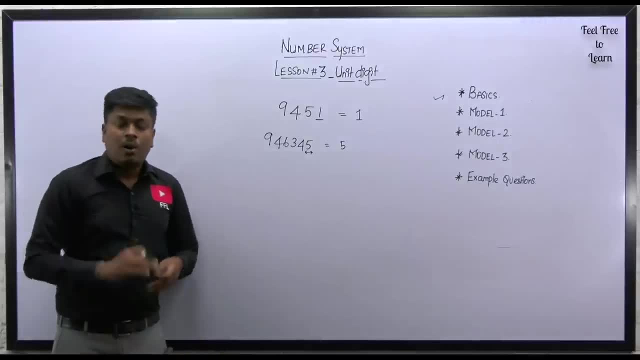 number. what you need to say? you need to say the last digit of the given number is five. So we can say that for the given number, the unit digit will be five Always. unit digit means the last digit of your final answer is called as the unit digit understood. So let me take some basic questions. 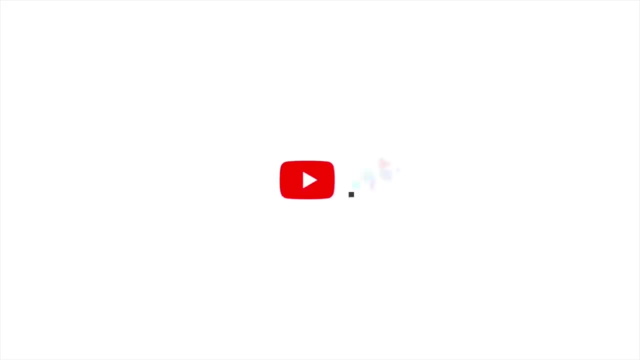 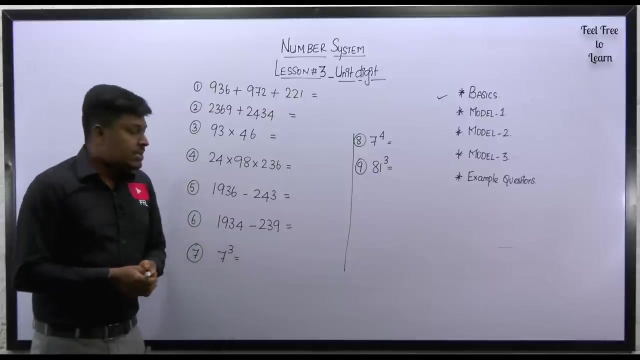 and we can learn the basics first. So here I have taken some example question that is basic level question. So initially let me find the unit digit for all these basic numbers, right? So first question: 936 plus 972 plus 221.. So our 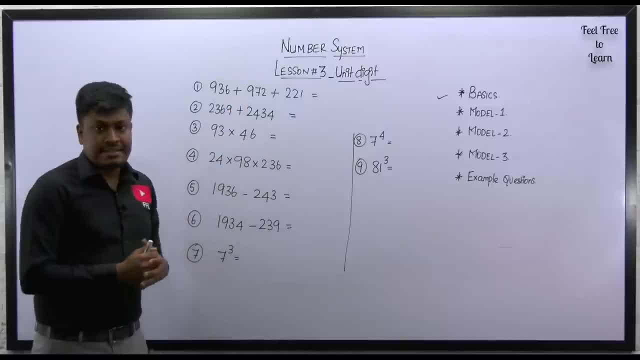 target is to find what is the unit digit of the final answer, right? So what is the unit digit? actually, just now I have told you unit digit is the last digit of the any number. just see here, you don't want to take any number, right? So what is the unit digit of the given number? 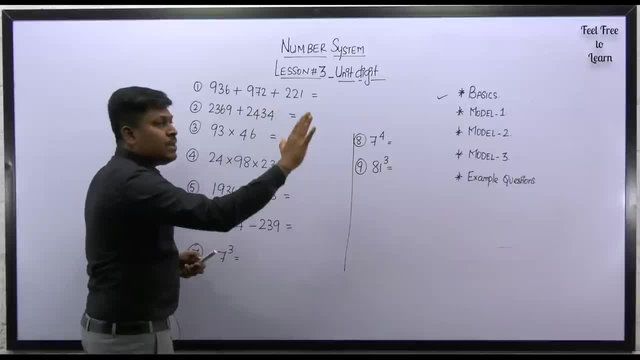 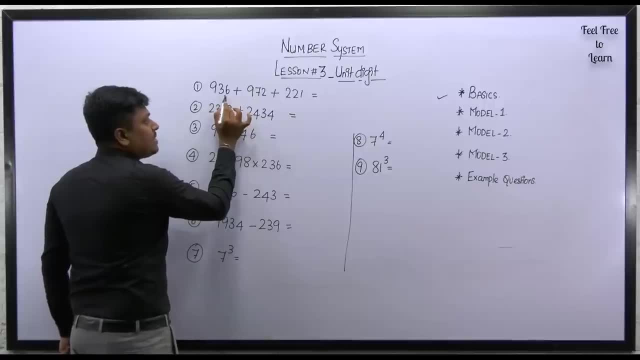 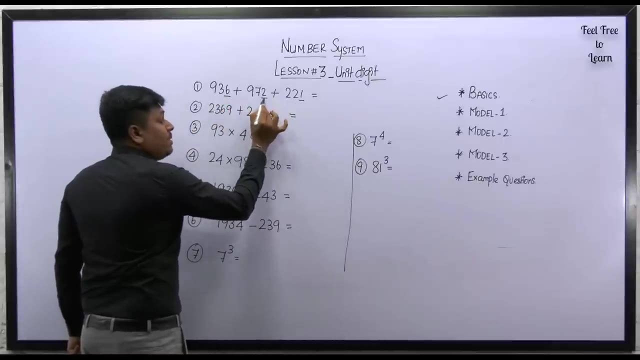 You don't want to add the complete number And then you don't want to find the unit digit. it is better to add only the last digit of all the numbers. See what is: the last digit of 936 is six, understood. So last digit is two. So last digit is one. So six plus two will be eight, eight plus one. 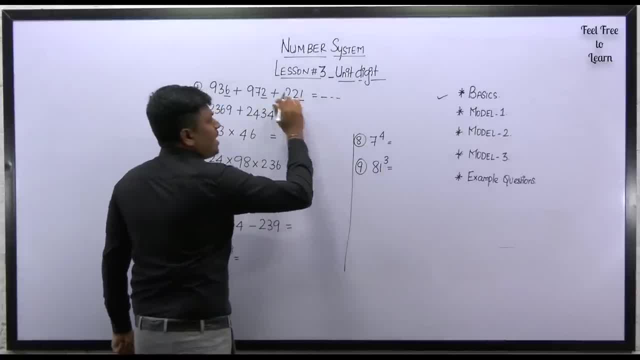 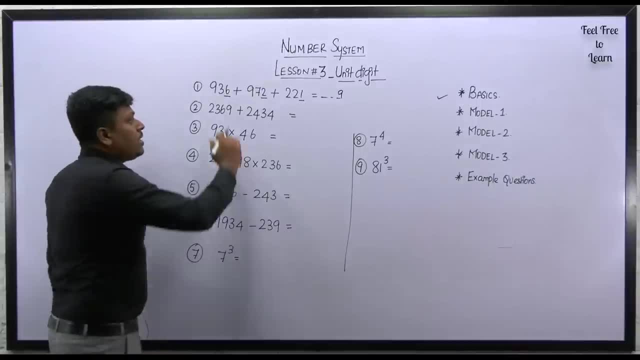 will be nine. So we can say that any number, it can be any answer, but that answer last digit will be nine. So, finally, we can say that the unit digit of the given number is nine. So we can say that the unit digit of this final answer is nine. So, friends, got it or not, right In case, if we need. 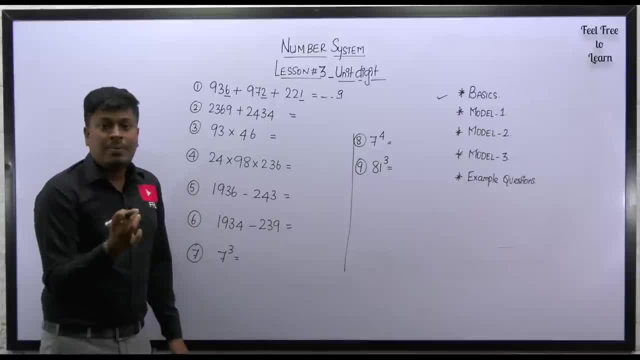 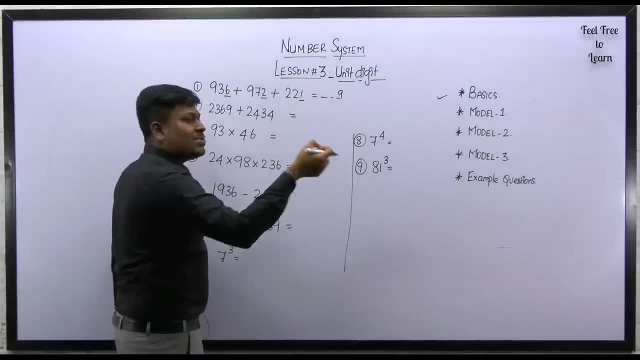 to find the unit digit of these numbers, then target only the last digit, because we don't want to find the first, second digit or nothing. Our target is to find the last digit that is called as unit digit. So it is better to add only the last digit alone, understood? So last digit is six. 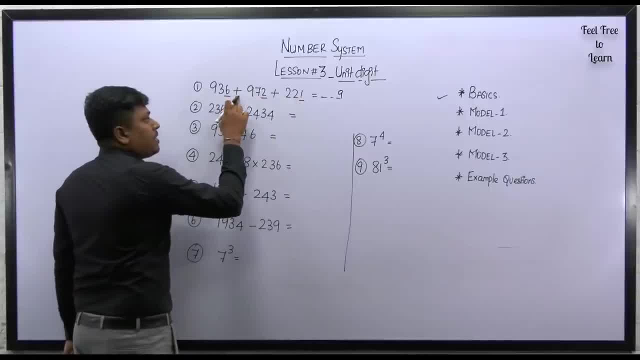 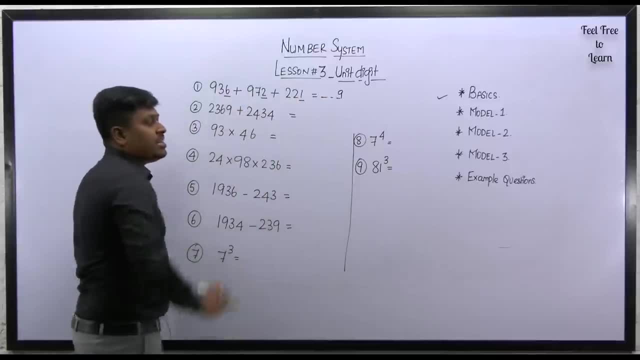 last digit is two year one, So six plus two plus one. So finally, six plus two will be eight, eight plus one will be nine. So finally, answer for this question number one will be nine, Understood friends. So second question: 2369 plus 2434.. So we need to find what is the unit digit. 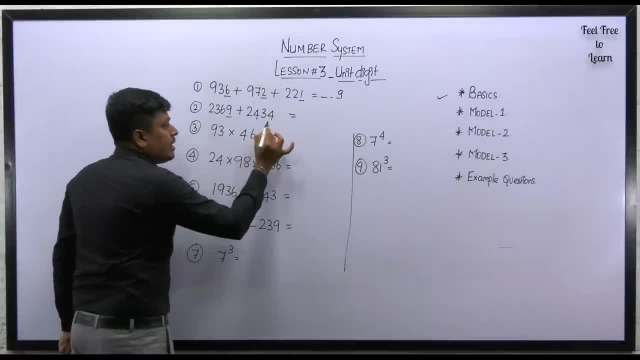 of the number. what is the last digit here is nine. What is the last digit here is four. So nine plus four is what 13.. Just listen carefully. we got two digit right, So 13.. Again, whatever be the last digit of the final answer is what? 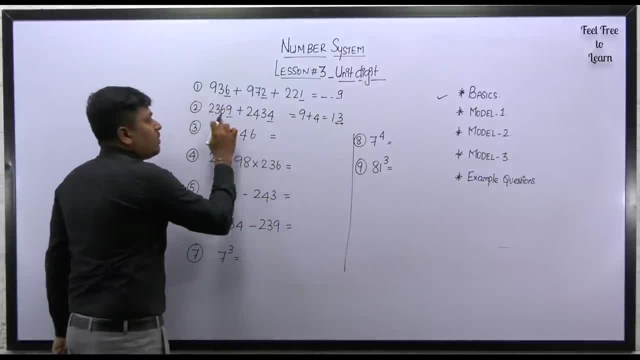 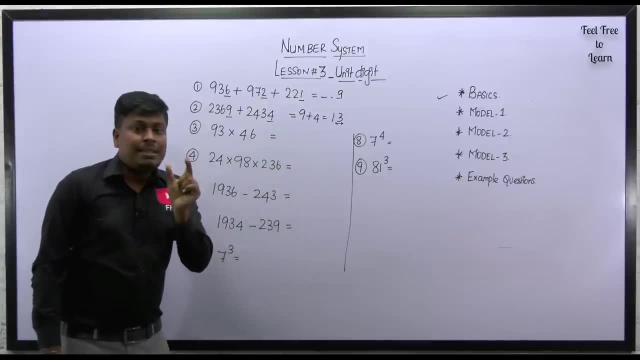 Three. So finally we can say that the unit digit of these numbers will be three, friends got it or not right? So nine plus four will be 13.. So in that number 13,. the last digit is three. So finally, 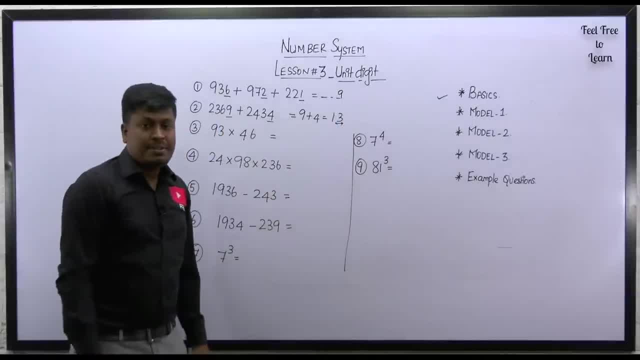 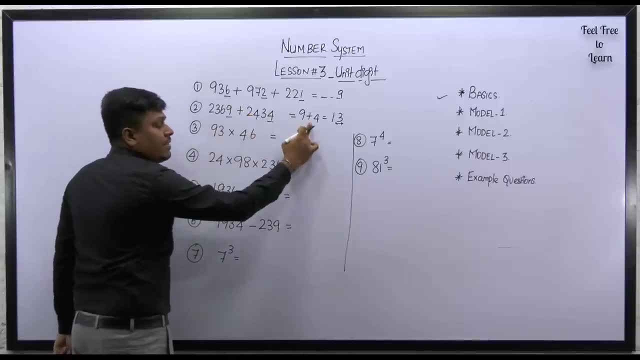 we can say that the unit digit of the final answer will be three. So let me move to the third question. So 93 into 46. See, here we have addition. So we have added. in case of multiplication we have to multiply, that's it right. So the last digit is three, the last digit. 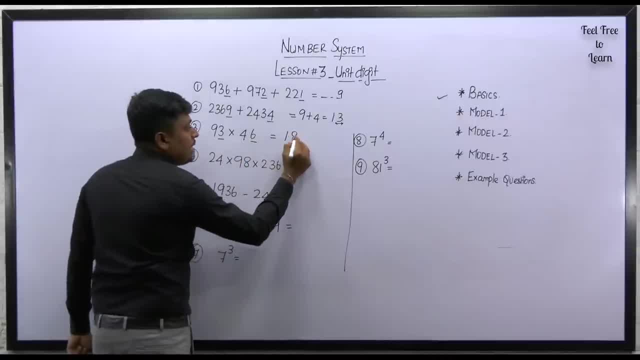 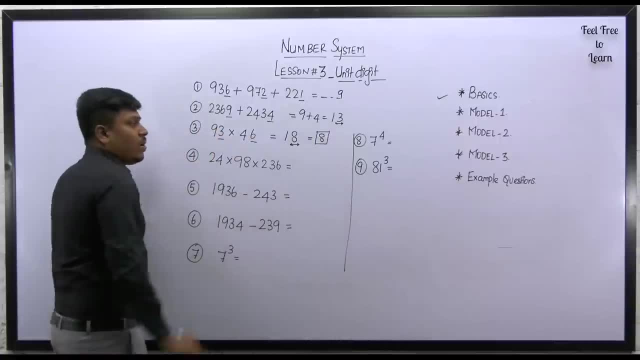 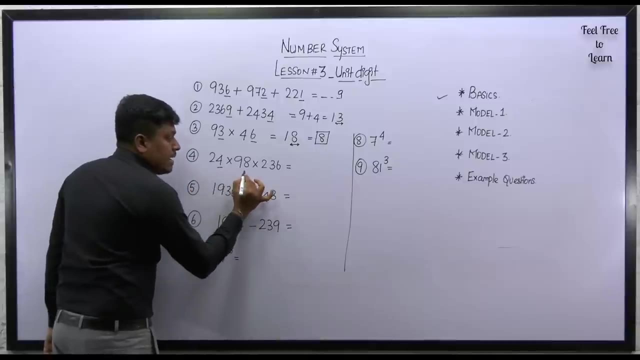 the last digit is six. six into three will be. is what? 18 got it. So the last digit of the final answer is eight. So we can say that eight will be the unit digit of question number three, So question number four, so 24.. So here we have 498.. Here we have 8236. is six got it? So we have. 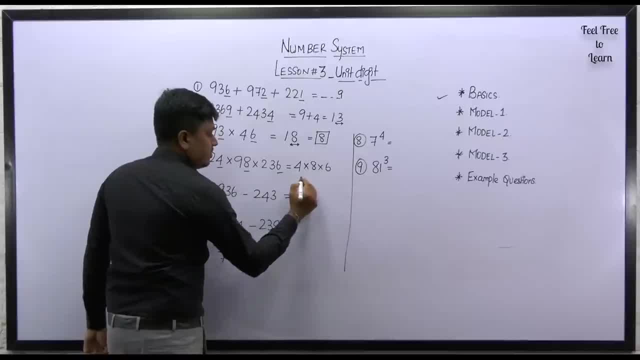 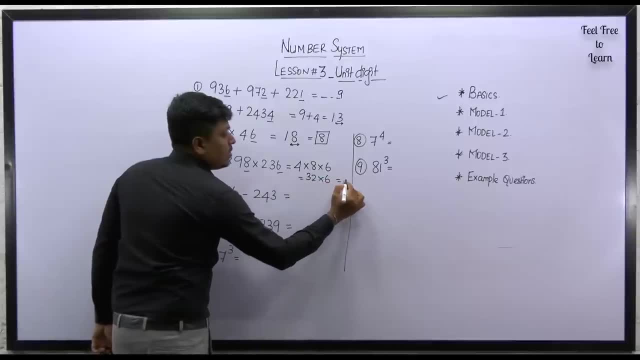 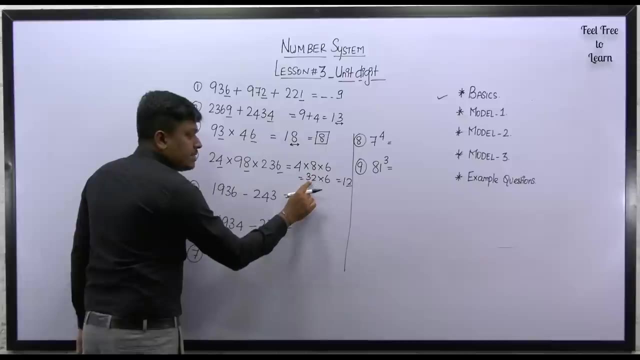 to multiply four into eight into six. So eight into four is 32 into six. So we have to multiply six. So six into two will be 12.. So the last digit will be two- friends understood what I did. So four, eight and six. So four into eight is 32.. Remaining we have six. again target the last number, So year. 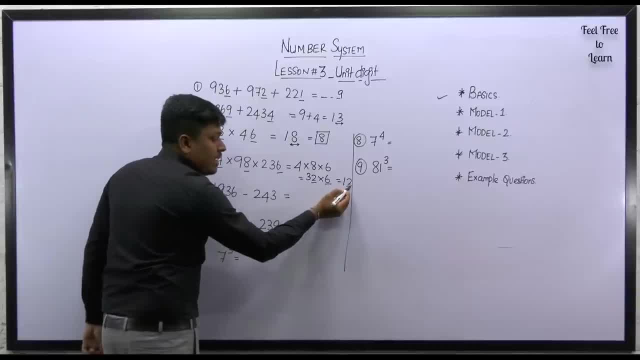 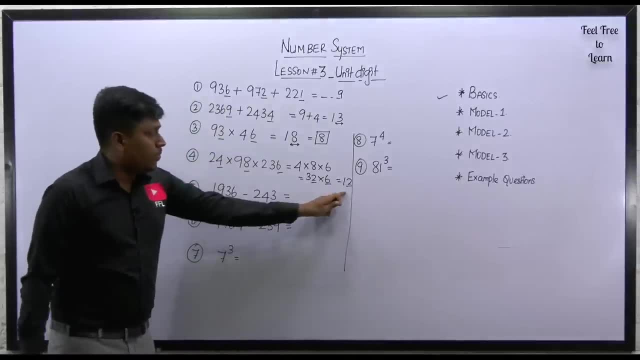 two year six, six into two will be 12.. So we can able to see the last digit of the final answer is two. So finally we can say that the unit digit of question number four is two, right. So next question: 1936 minus 243.. 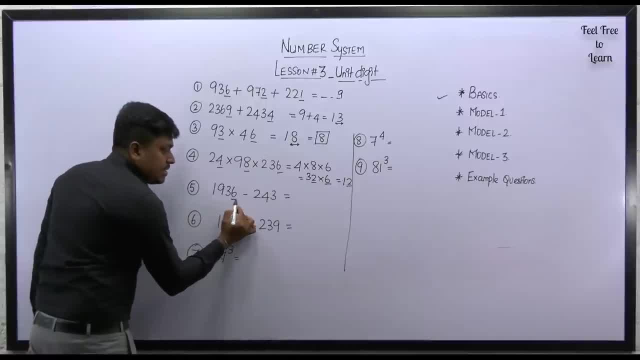 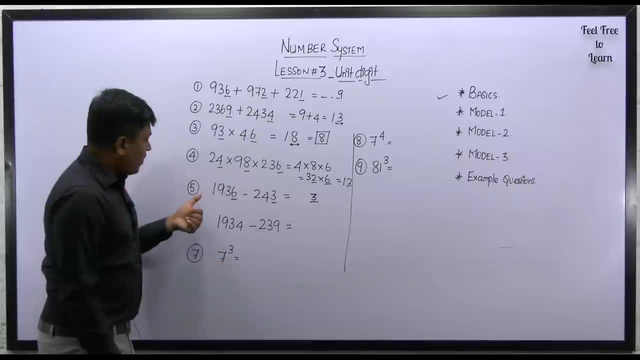 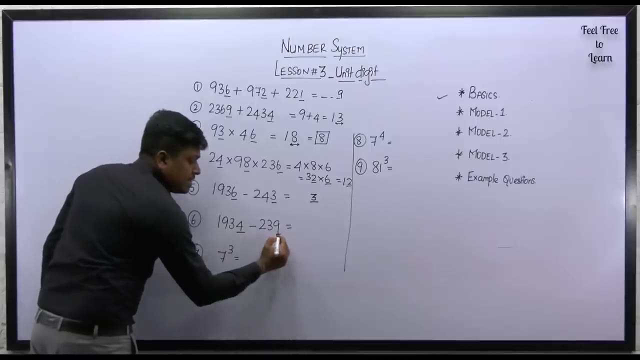 Listen here. here we have subtraction right. So the last digit is six, the last digit is three. six minus three is three. So finally we can say that the unit digit of question number five is three. So question number six, the last digit of the given number is four And the last digit is: 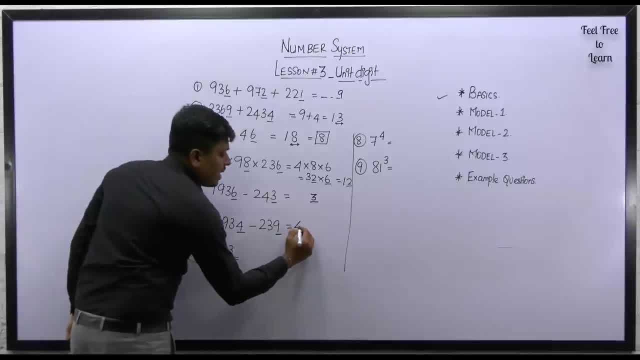 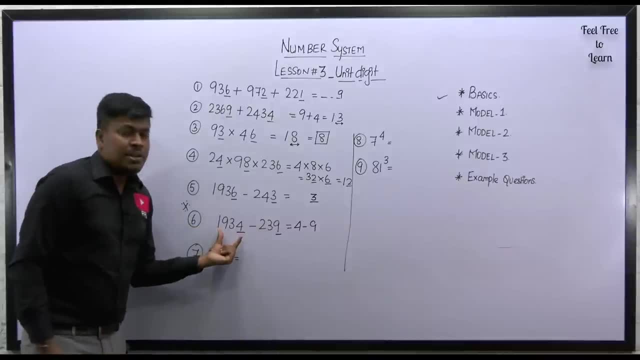 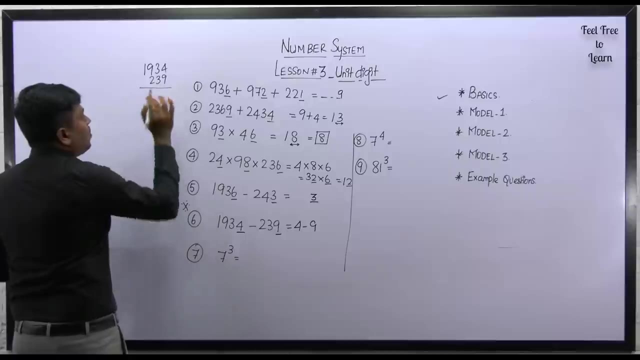 nine, Most important, just listen here. So we have to subtract four minus nine. you should not write it as minus five. That is wrong actually Why? Because usually, how will you subtract? usual process? We can see: one, nine, three, four. right, We have to subtract with 239.. How usually you will subtract? 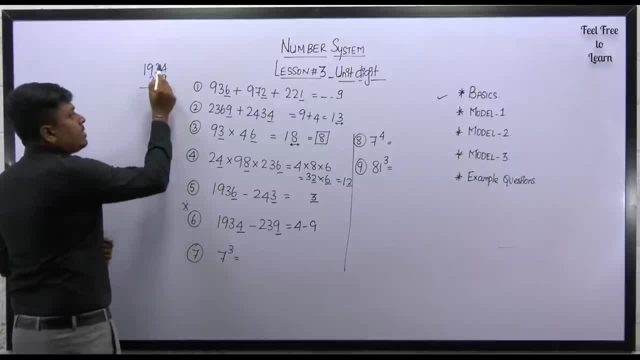 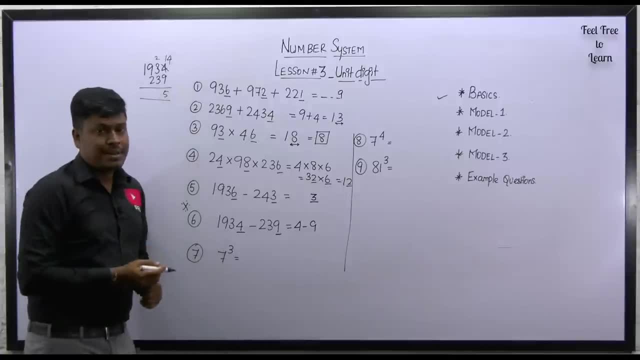 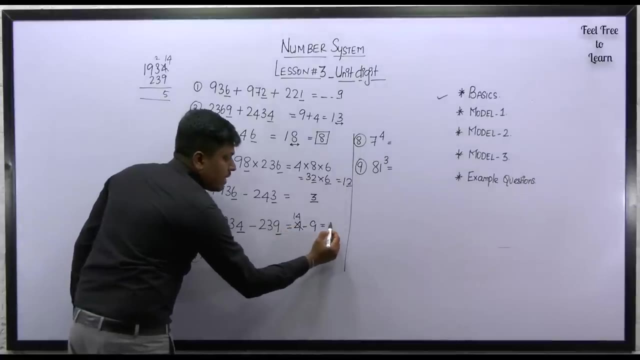 in the exams. So here you have four and nine right. So usually you will write it as 14. carry one, Yes or no. 14 minus nine will be five. This is the way we used to calculate Similar process. So four minus nine we have to subtract. cancel it 14 times. 14 minus nine will be five. So finally, 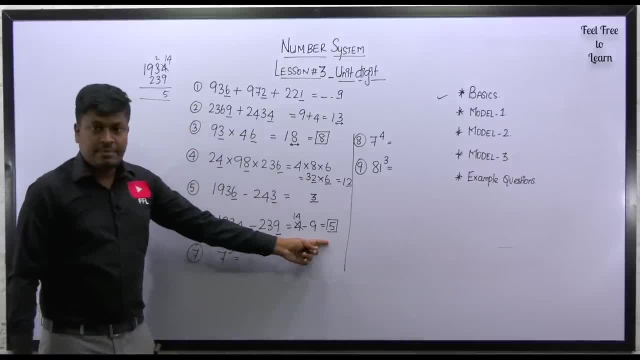 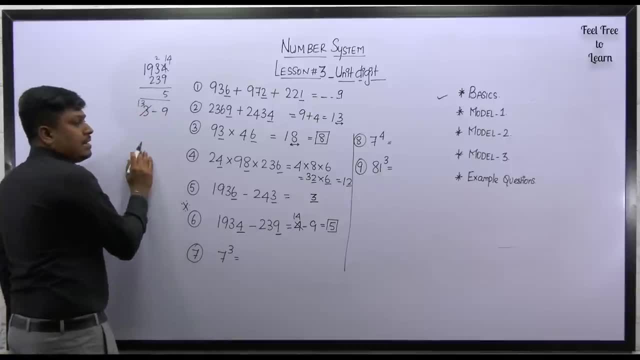 the unit digit of the final answer will be five. So friends understood, if it is three minus nine, what do you do? What do you have to do? three minus nine? So first you have to write it as 13 carry one got it So. and then 30 minus nine you have to. 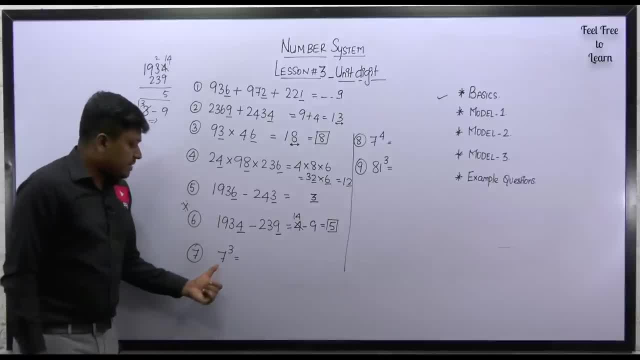 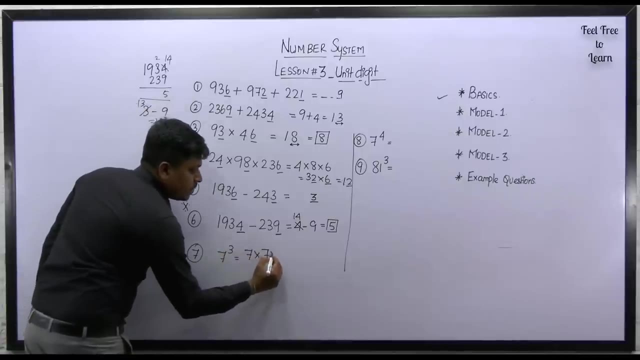 write the remaining answer Understood. So question number seven: seven cube. just listen here. important question: seven cube. So if you, if you know the answer- 343, that is okay. In case, if you don't know what is the answer of seven cube, what you need to do is write as seven into seven into seven. 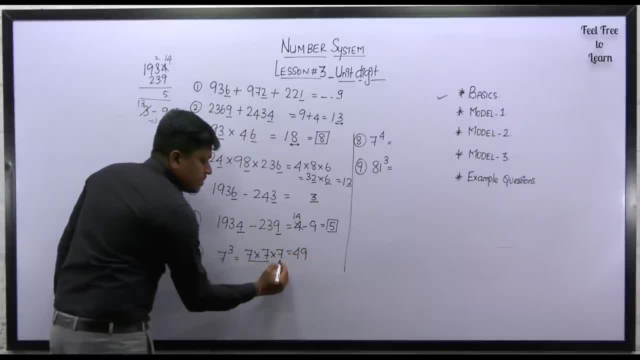 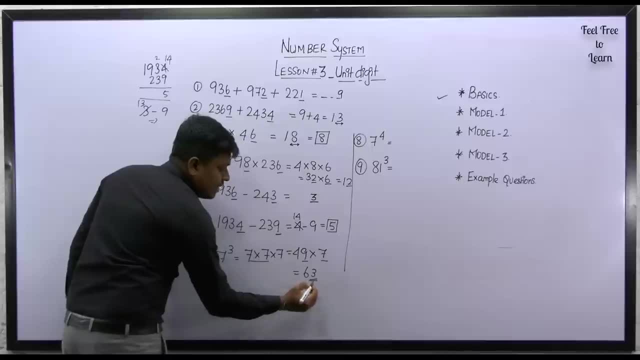 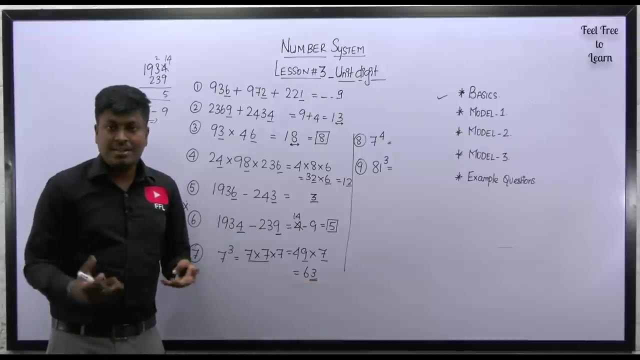 Got it. Seven into seven is what 49, right? So reminding that we have a seven multiply the last digit, nine into seven, is 63. So, finally, the last digit is three. So we can say that answer for this question: the unit digit of this number is three. Everyone's understood, or not right? 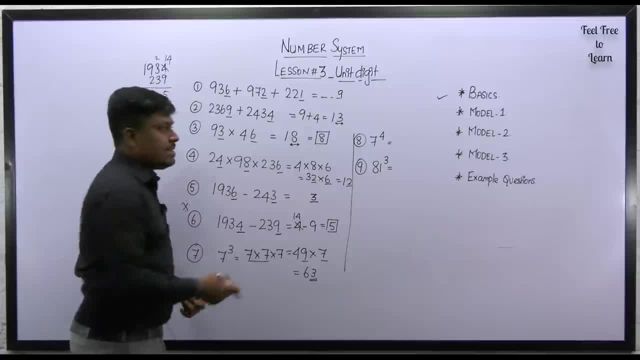 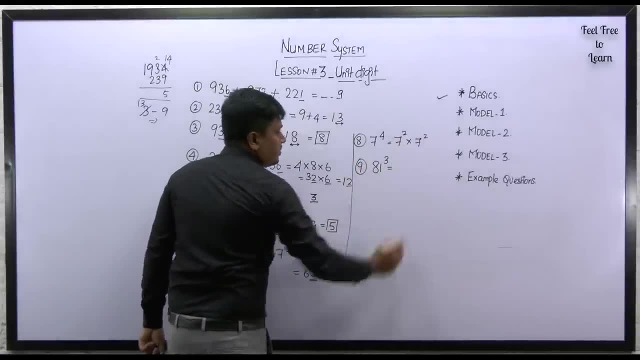 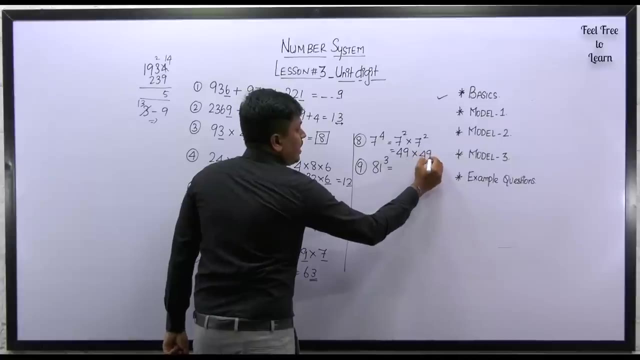 So question number eight: seven power four. just see here: seven power four. how we can convert the seven power four. we can write this as seven square into seven square. Got it Easiest way. What is seven square, Seven square is what 49.. So 49 into 49.. Got it, So now multiply. 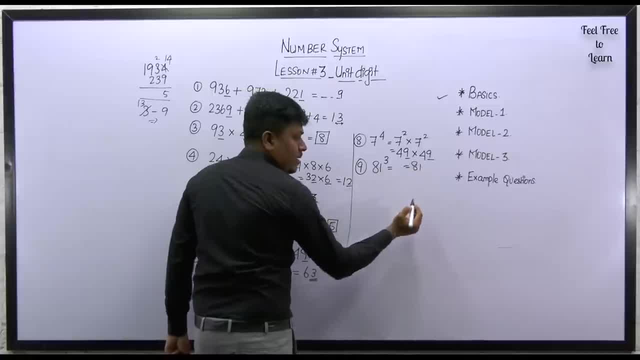 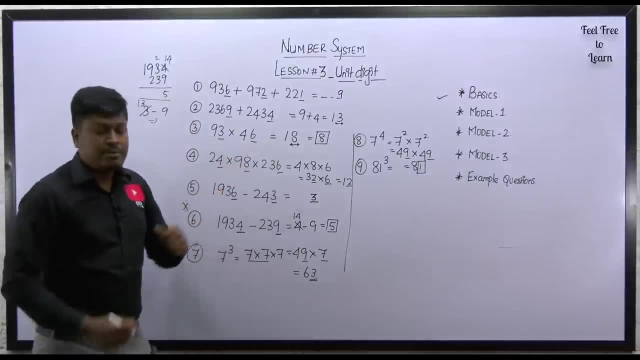 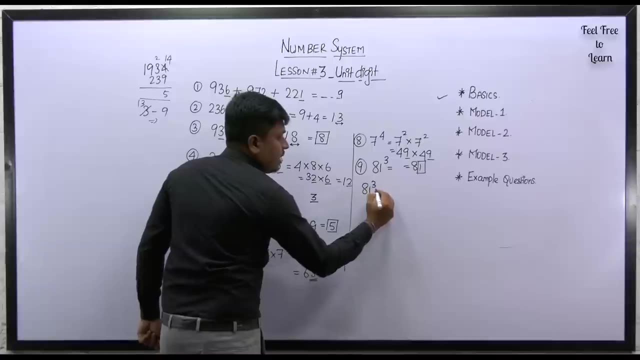 the last digit, nine into nine, will be 81.. So we can say that the last digit will be one. So we can say: unit digit of seven power four will be one, Understood. So last question, number nine. So question number nine is what 81 cube, right? So 81 cube can be written as 81 into 81 into 81. 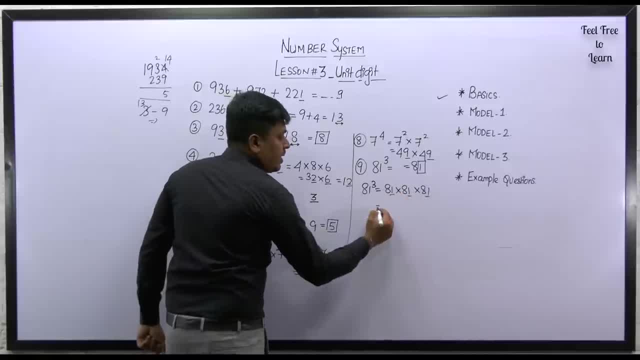 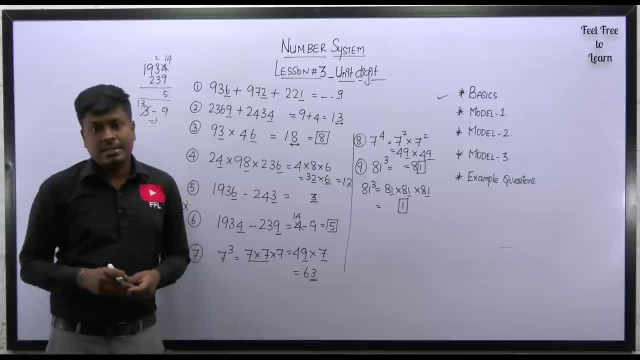 So last digit of all the number is one. we have to multiply So one into one, into one so one. So finally we can say that the last digit, that is unit digit of 81 cube, will be one. So once initially we have learned the basics, it is easy right? So every time in case, in the exams, 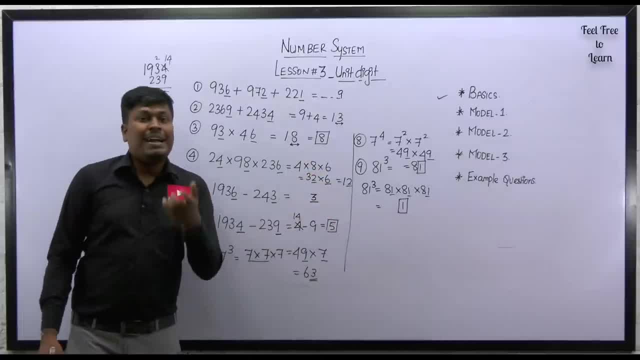 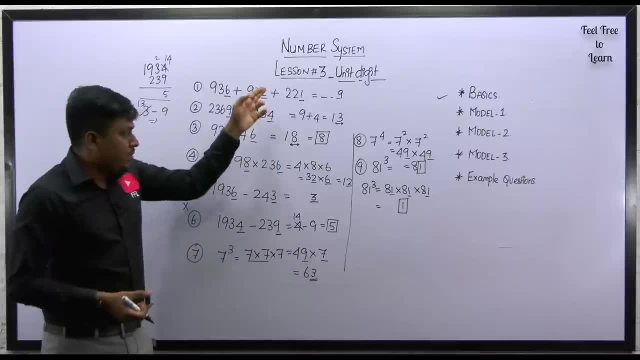 if they ask to find the unit digit, you don't want to find the complete answer. it is better only to find the last digit of the answer. right, That is called as unit digit. So everywhere you can able to see, we have found only the last digit Understood, So only one. 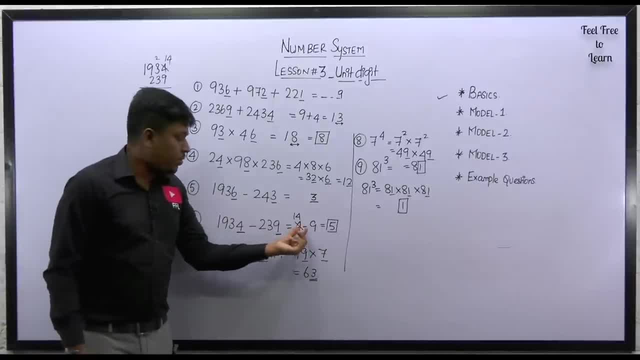 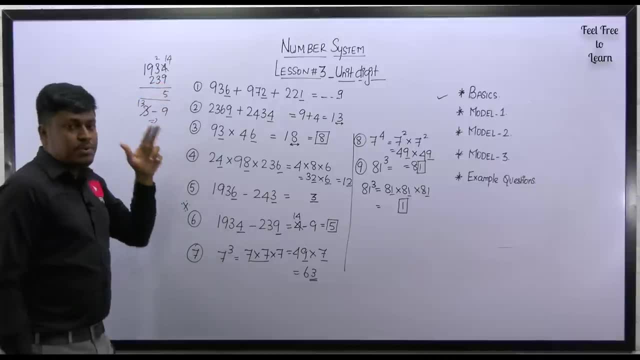 important thing. don't make mistake here. most of the students will write as four minus nine, as minus five. that is wrong. Actually, how will you subtract If the last number is four? here, last number is nine. usually what we do in the exams, we will cancel it as 14, carry one and 14.. So here, 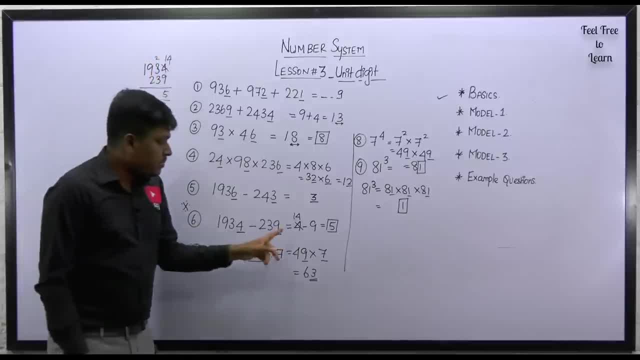 already two. So 14 minus nine will be five. So similar process I have done: 14 minus nine will be five Understood. So now let me move on to all the models. So let me move on to all the models. 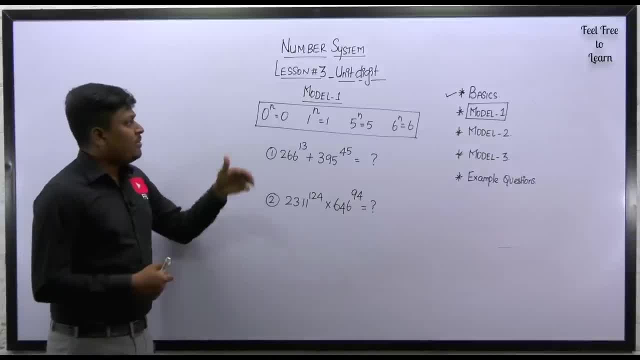 Now you can able to understand the concepts. So let me move on to this model number one. So in this model number one, initially we are going to learn the unit digit for some important numbers. that is easy to remember: zero power n. Example: if it is zero power, anything for zero power, 99, or zero. 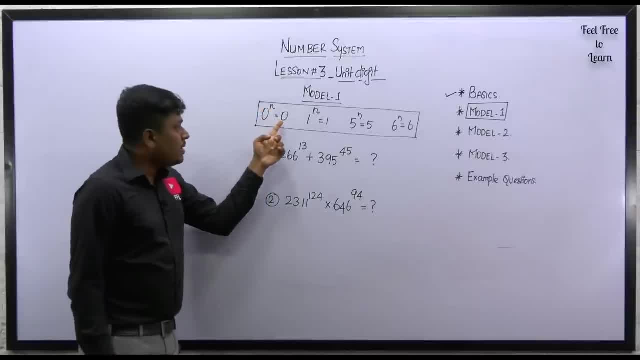 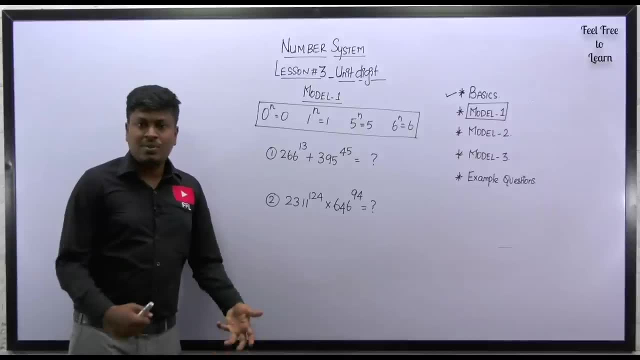 power 23,. anything power zero right is called a zero. Similarly, one power n is one. five. power n is five. six power n is six. So in this model we are going to learn the unit digit for some important numbers, that is six. So, friends, got it or not? Just see example. for example, let me take any. 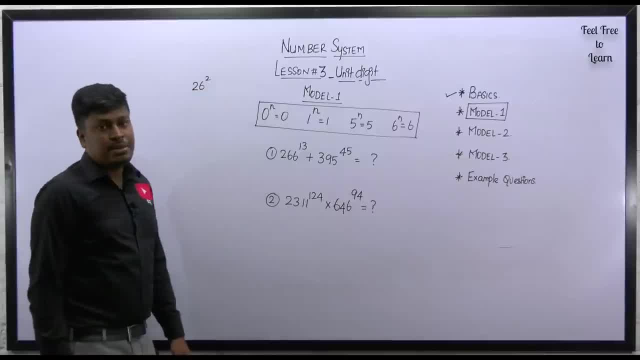 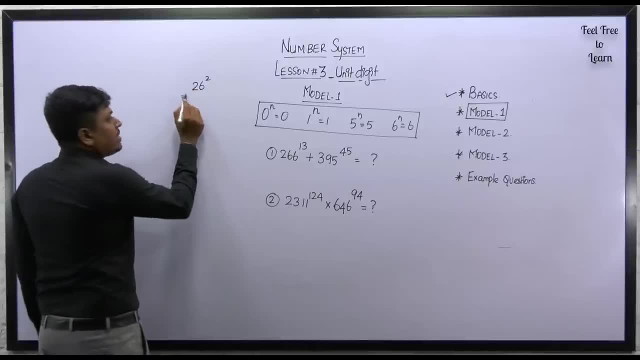 numbers 26 square, right, Let me take this number, 26 square. So we have to find what is the unit digit for 26 square. it is easy to find for 26 squares or no? you can write this 26 as 26 into. 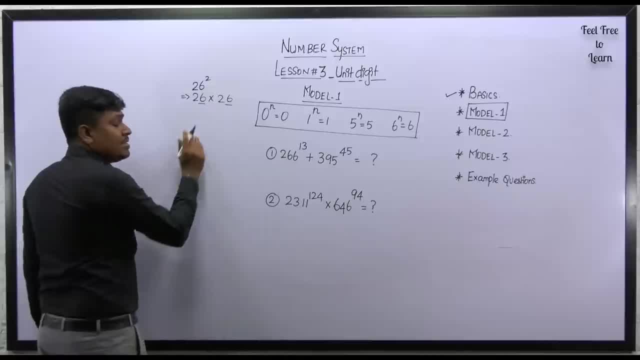 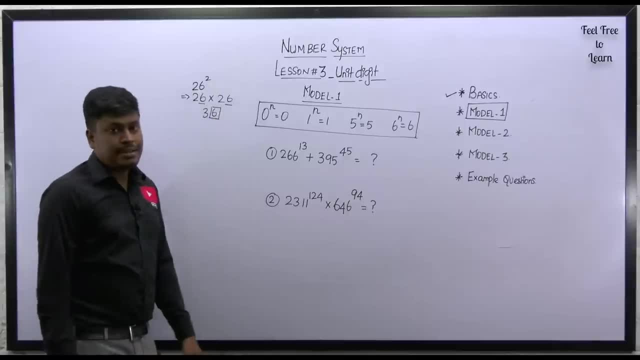 26.. Got it. So last digit is six, last digit is six. So six into six will be 36.. And the last digit will be six here. So finally you can say that the unit digit will be six. So you can say: 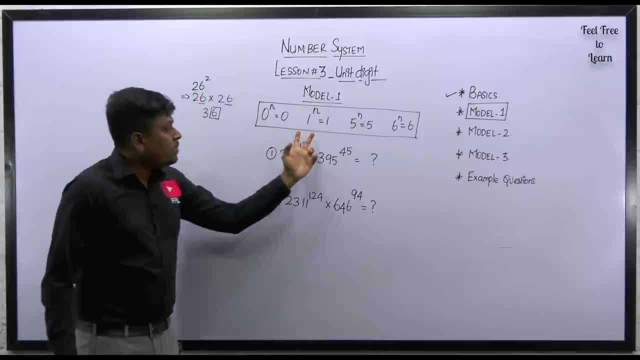 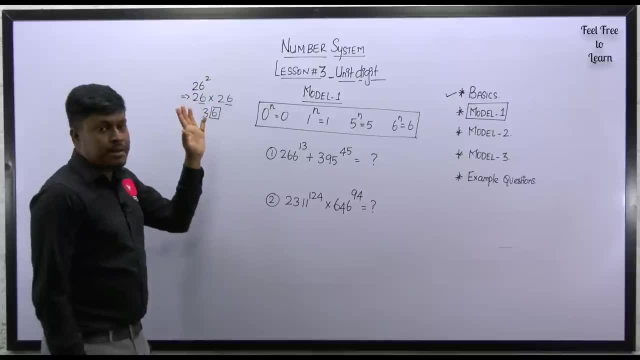 that the unit of this 26 square is six. But according to this logic, instead of finding all these stuff right, we can directly say: six power any number. it can be n, so just see six power any number where the unit digit will be six. you don't want to find it. six power anything. the. 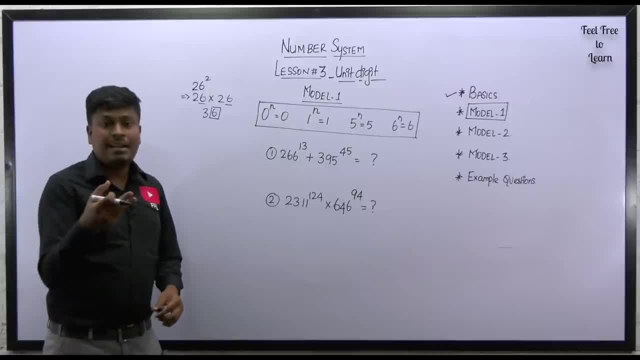 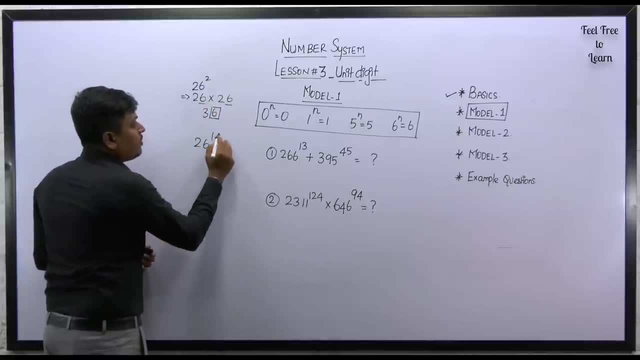 unit digit will be six. And another important thing is: in the exams they won't ask you an easiest number. see, they won't ask you 26 square. they will ask you like 26 power 142. Is equal to question mark. finding us easy or not? it is very difficult If you go with 26 into. 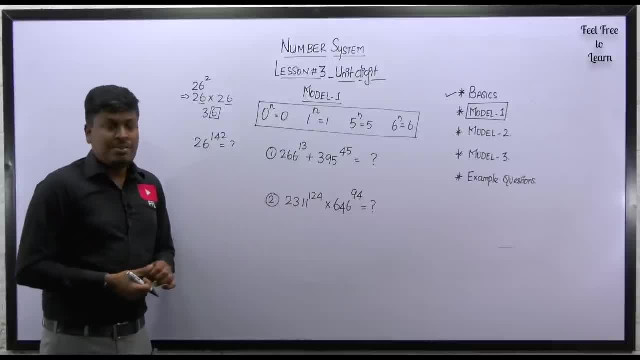 26 into 26,. it takes a lot of time right. So that's the reason we are learning all these tricks: to solve this question. Just see here: the last digit is six and the power is 142.. Just now we. 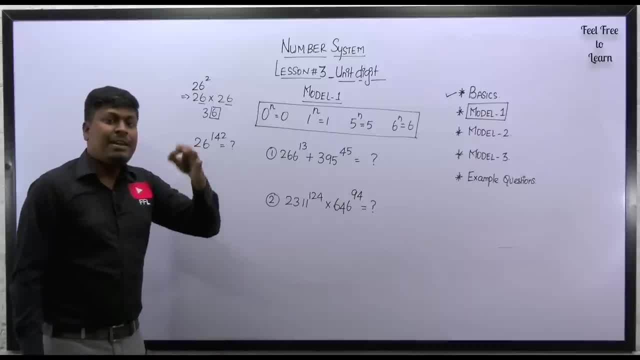 have learned six power- anything right. Six power: n any number. six power: the resultant last digit will be six. So that's the reason we have learned in this model number one. we are going to learn One power: anything is one. five power: anything is five. six power: any number will be. 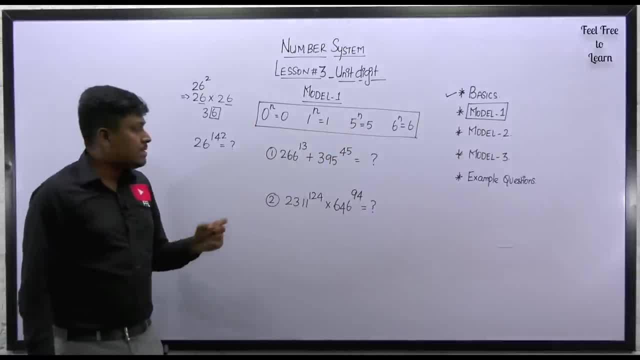 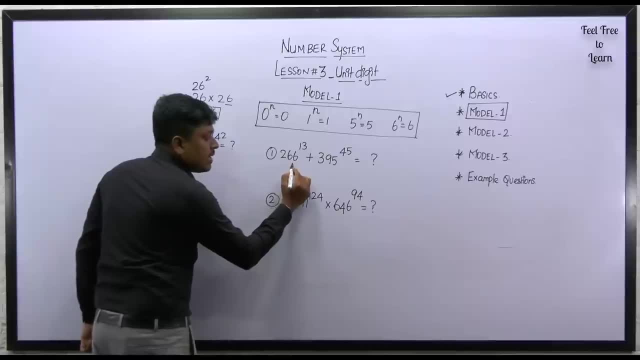 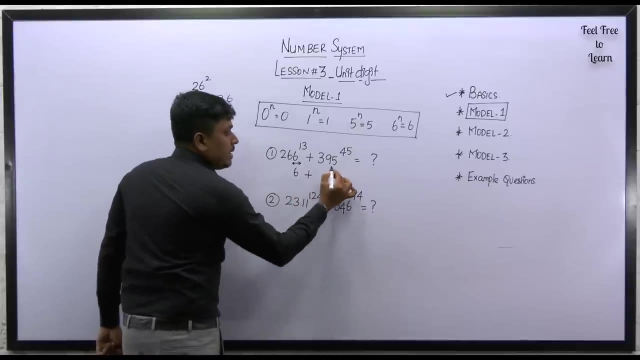 six. So here I have written some example question. just see here: 266, power 13.. So what is the unit digit? So here you can able to see 266, the last digit is six, six, power, anything. definitely. the resultant answer will be six, So plus here. the last digit is five, five, power, anything will be. 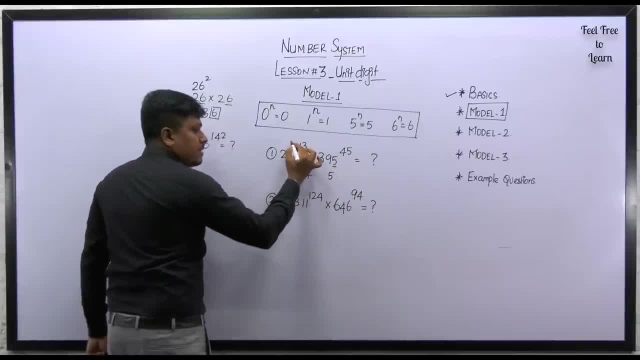 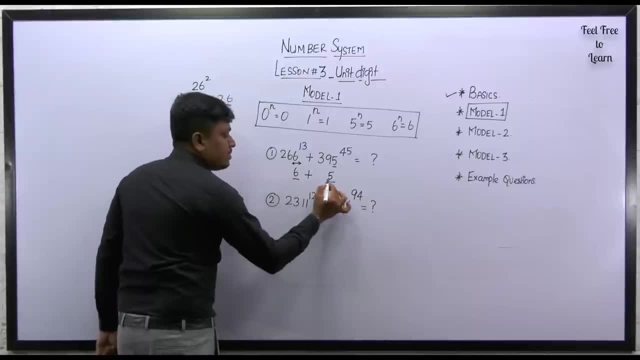 five. So finally, if you multiply all these numbers, the final digit will be six. Similarly, if you multiply and find, the final answer will be five. So six plus five will be 11.. So finally, we can say that the unit digit of the first equation is: 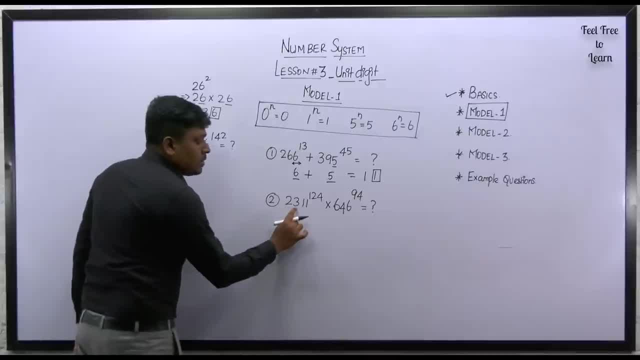 one. Friends understood right. So next, 2311, power 124, into 646, power 94.. Just see here, the last digit of 2311 is one one power. n one power. anything will be definitely one. So the last digit is one one power. anything will be definitely one. So the last digit. 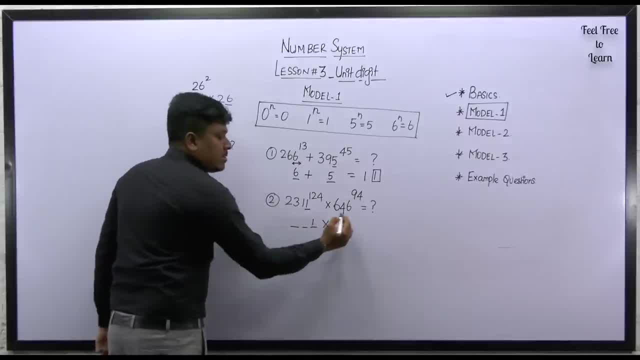 of this answer is one understood, So multiplication. so here the last digit is six. six power, anything will be definitely six. So the last digit will be six. So one into six will be six. So finally we can say that the unit digit of this number will be six. So this is the thing. 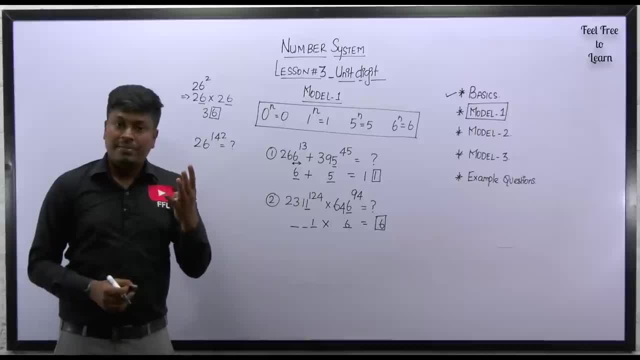 we have learned in this model number one. Model number one, totally, we have four numbers: zero power, anything is zero. one power: anything is one. five power: any number is five. six power: any number is six. So friends understood. So this is model number one. we, in this model number one, we have learned: 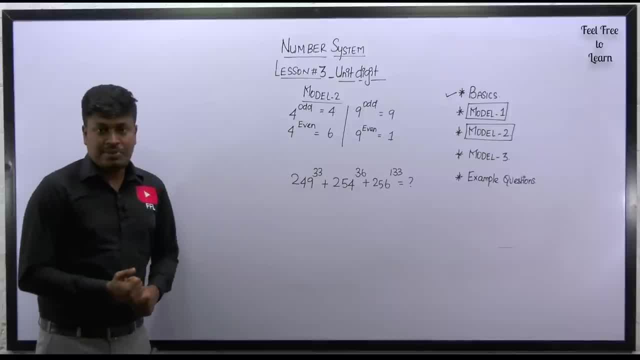 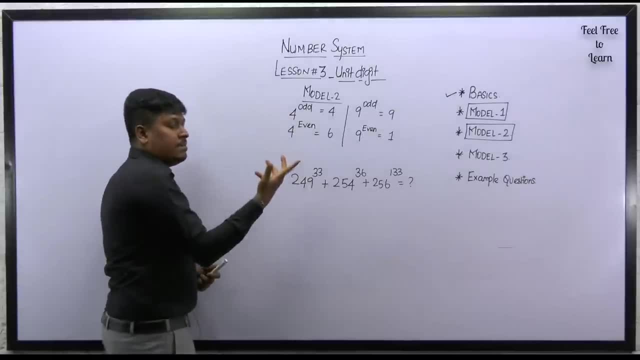 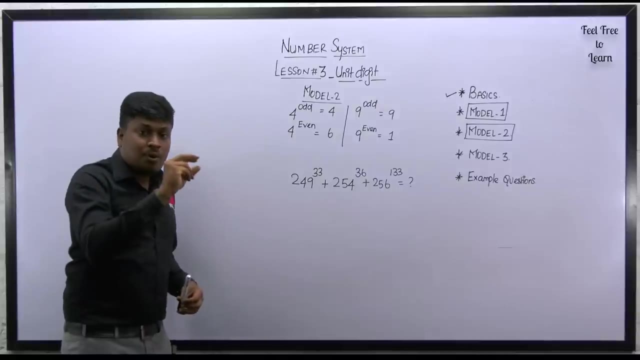 for four numbers. So next model. So in this model number two, we are going to learn for this two numbers, that is for four and nine. Just see here: four power odd number right. Four power odd If it is four power 23,, four power 25 or four power 33.. So four power odd number. So the resultant. 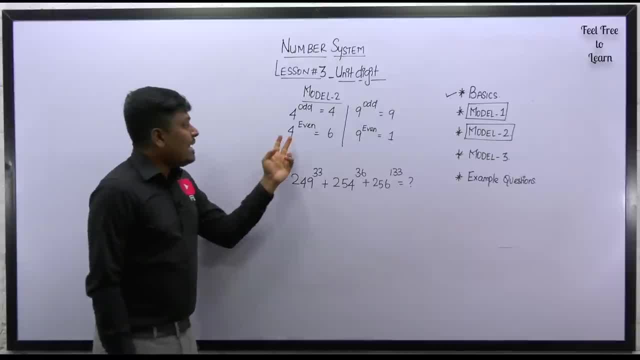 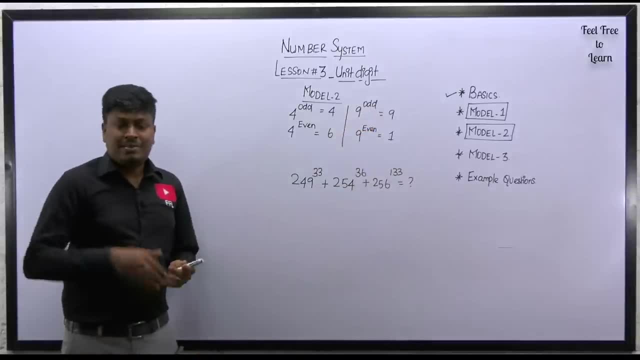 unit digit is four. Similarly, four power even number will be six. So nine power odd number will be nine. nine power even number will be one. So got it So easy to remember: four power odd number will be four. nine power odd number will be nine. four power even. 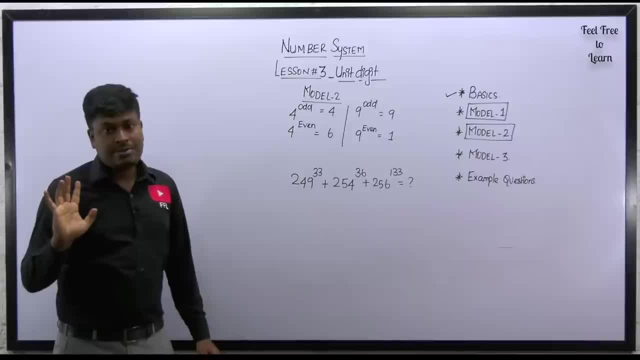 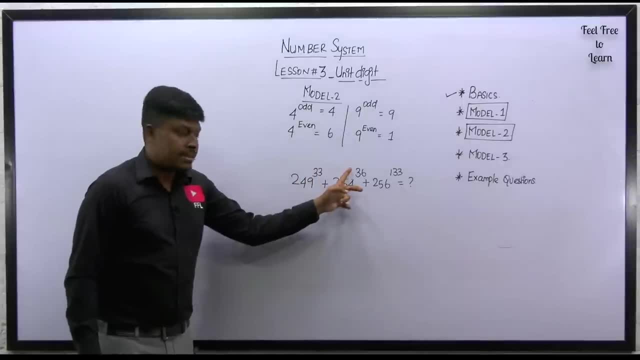 number will be six, nine power even number will be one Understood. So let me take one example question. Just see here: 249 power 33,, 254, power 36,, 256, power 133.. So we have to find what is the. 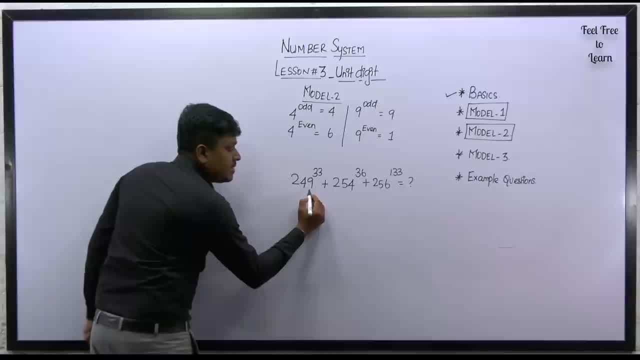 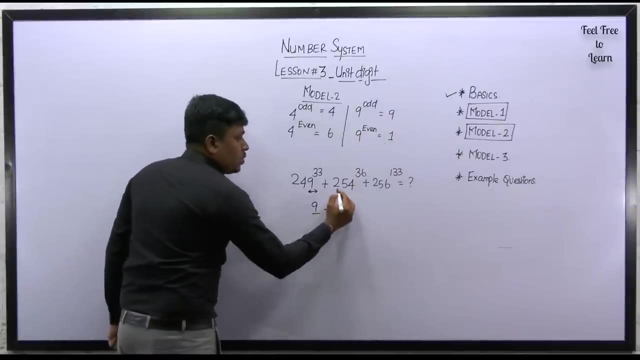 unit digit of the final answer. Just see here The last digit: 249 is what Nine, right? So nine power 33, nine power 33 is odd or even 33.. 33 will be odd number, So nine power odd number. resultant unit digit will be nine. So plus 254 power 36.. You. 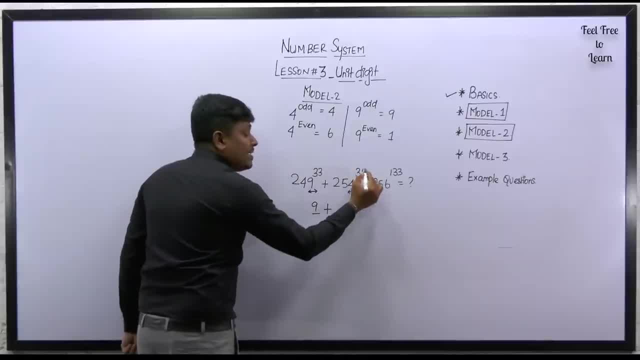 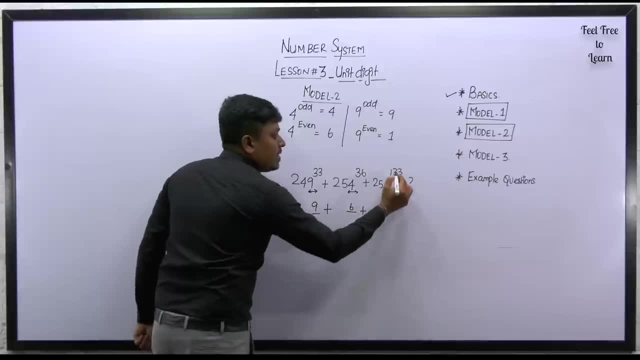 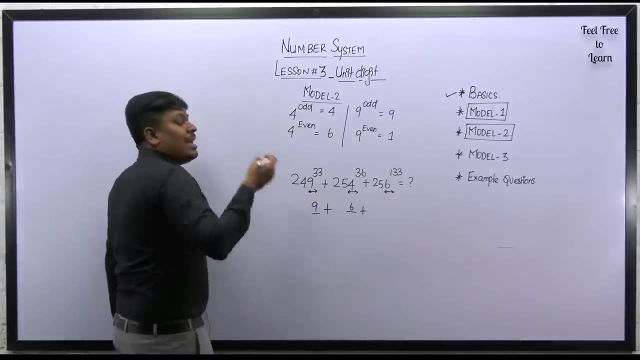 can see: last digit is four and the power is 36.. So four power even number. four power even number. the last digit is six Plus 256 power 133.. Just see here: the last digit is what Six Just know we have learnt in previous model. if a number that ends at 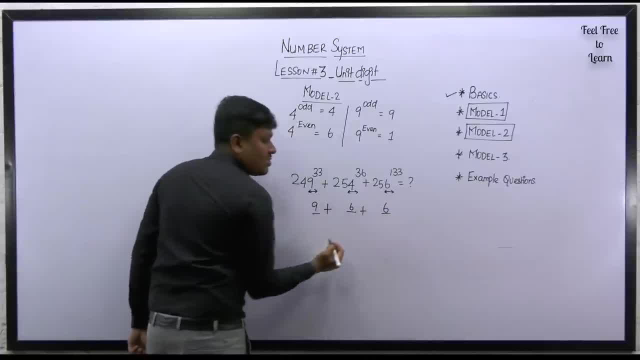 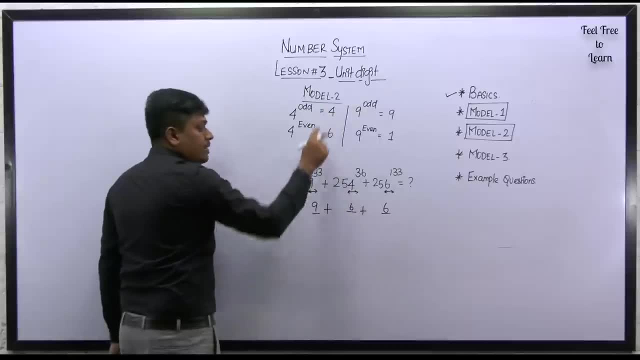 six, six power, anything will be definitely six, Understood or not. So last number is six. This is the thing what we learnt in the previous model. So nine and four we have learnt in this model, number two. So now we got the last digit of first number, nine, last digit of second number, six. 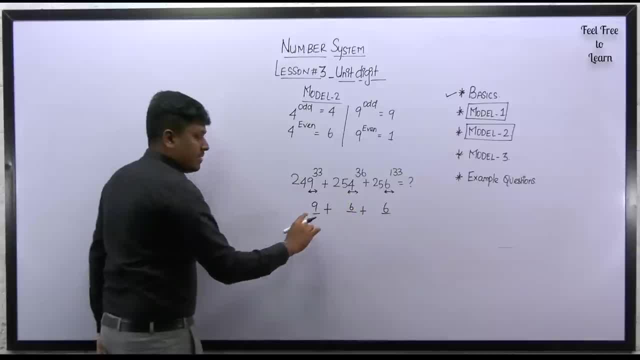 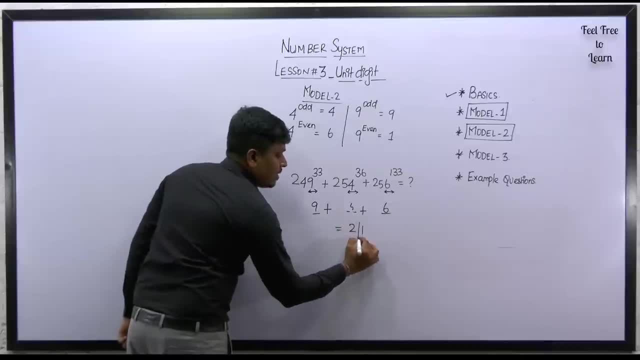 last digit of final number is six. Now we need to add all the stuff. So nine plus six will be 15.. Six will be 21.. So we can say that 21.. So here the last digit is one. So finally we can say that. 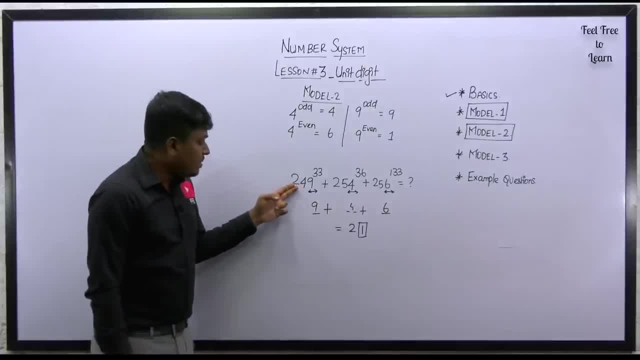 the answer for this question. the unit digit of this given question will be one. So friends understood right. So in this model number two we have learnt for two numbers, that is, one for four and another for nine. That's already. we have learnt for zero, one, five and six. Now we have. 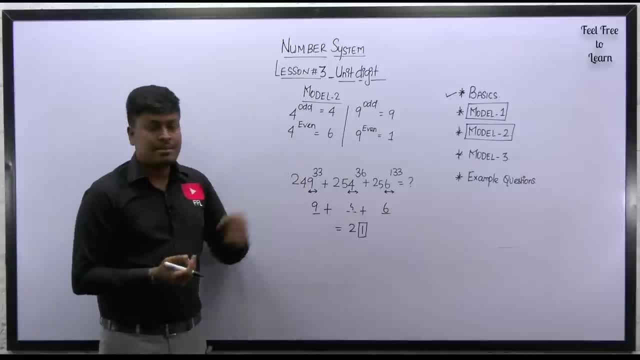 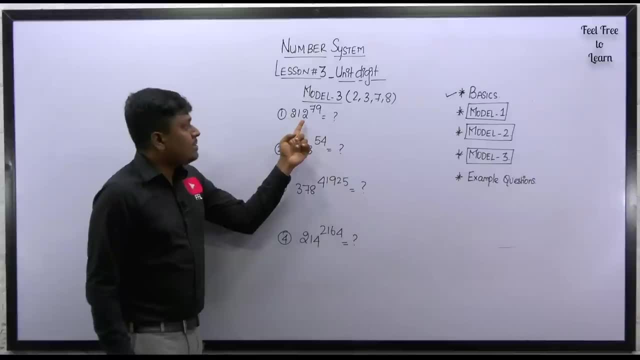 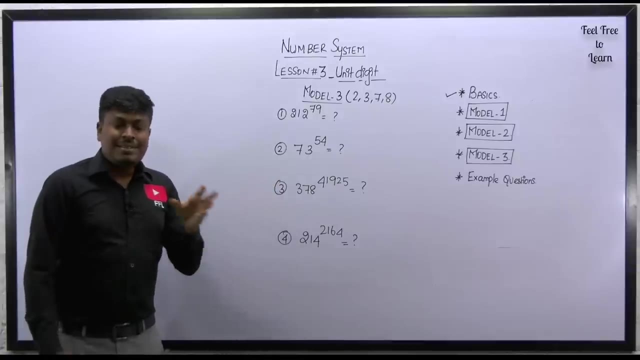 learnt for four and nine. So finally, we will be learning the remaining numbers in model number three. So model number three, we are going to learn if the last digit that ends at two, three or seven and eight. So this model is a different case. you have to learn something newly. Just listen here. If 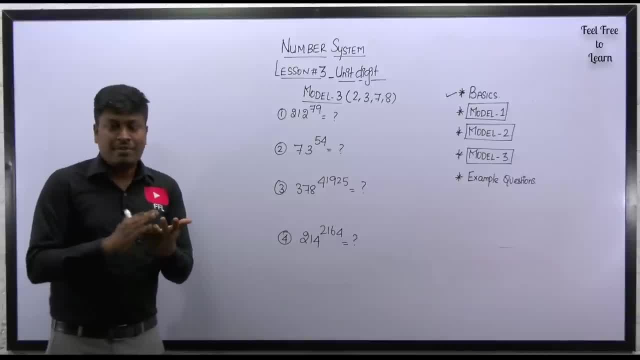 model number one. model number two is easy, right, We have a shortcuts. But in model number three alone, if you find the last digit, it is two or else three, or else seven or eight. what you need to do is you need to divide the power by four, a base number. 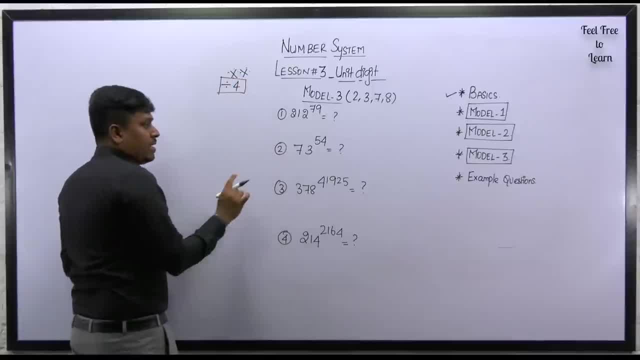 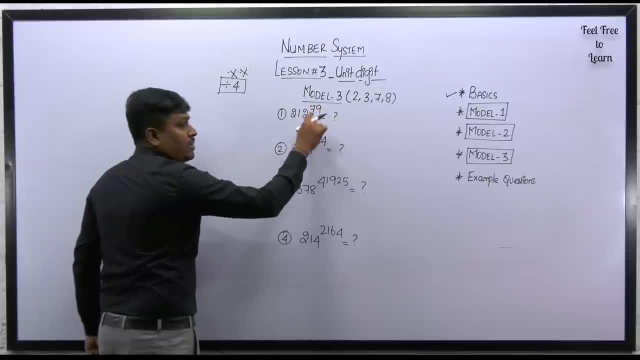 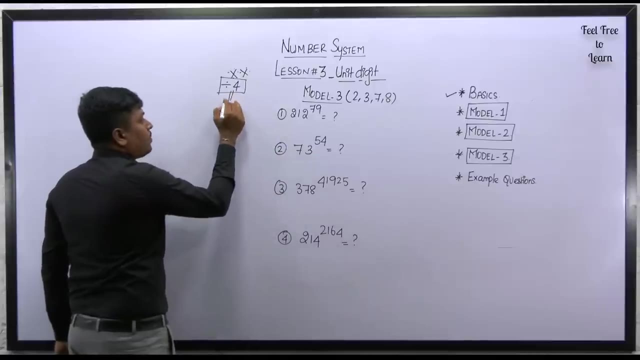 This is most important. So always remember that if a number that ends at two, three, seven or eight, you have to divide the power, right power of the given number by four. and got it. This four is the base number. you have to divide by four And you have to find the reminder, Got it. 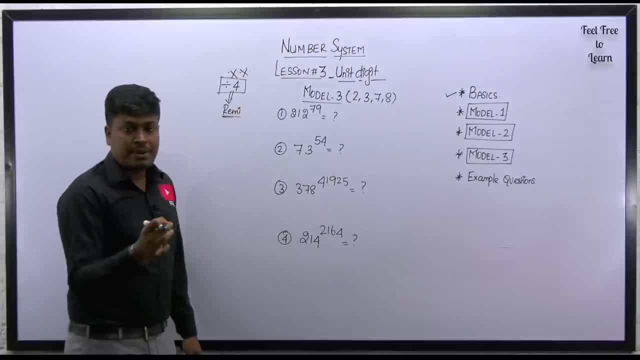 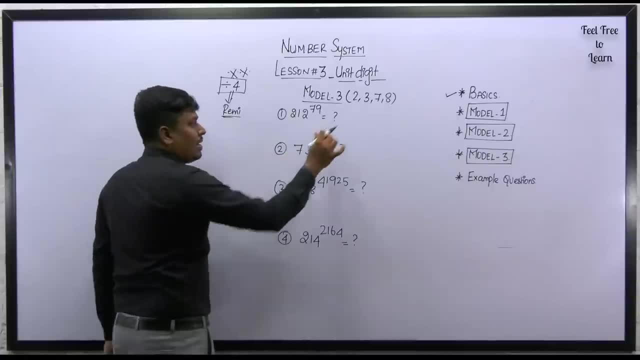 Got this step or not. You need to divide by four and you need to find the reminder. Next step: I will tell you what you have to do. Just see here: Two hundred and twelve, power 79, Step number 1, just see what is the last digit of this number: 212,. last digit is 2.. 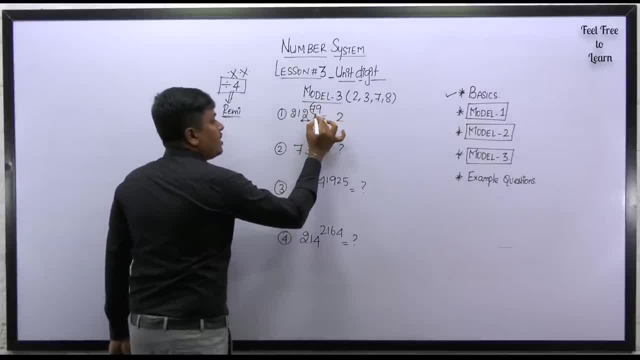 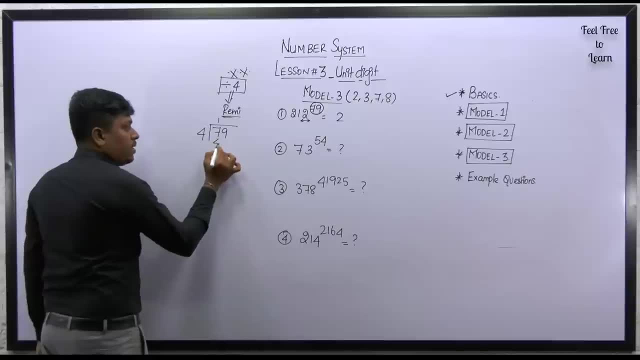 So now what you need to do is just see the power. what is the power here? So power is 79,, so 79,. divide this 79 by 4, got it. So 1, 4's are 4, so 4 here. remaining will be 3,, 39,, 9, 4's are 36, remainder is 3.. 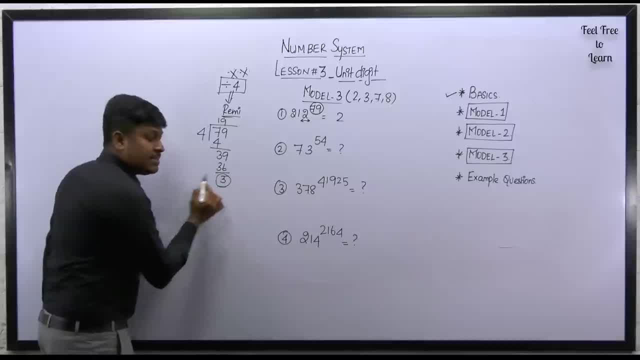 Just listen carefully. what is the remainder here? Reminder is 3, just now I have told you you have to divide the power by 4 and you need to find the remainder. So what is the remainder we got is 3, so put the remainder 3 here, got it. 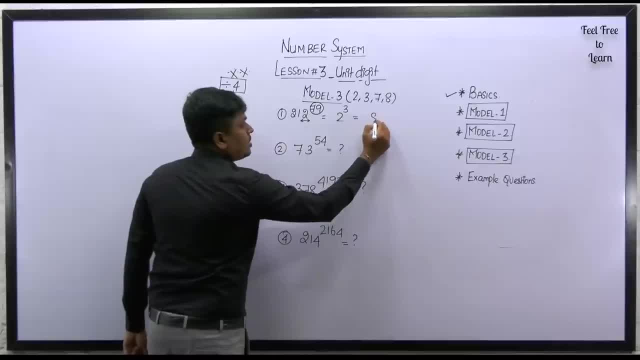 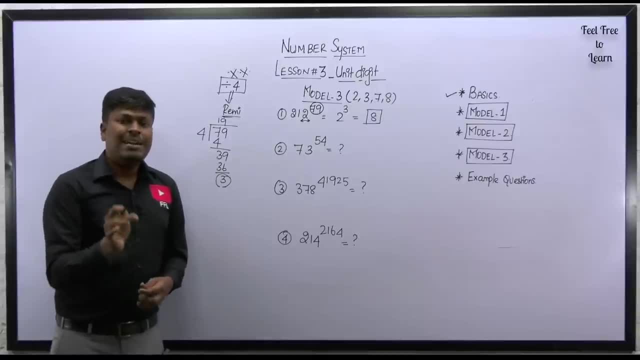 So 2 power 3, 2 2's are 4, 4: 2's are 8, so we can say that the unit digit of the number is 8.. So, friends, understood or not? Initially, first time, if you are learning, understanding is little bit difficult. 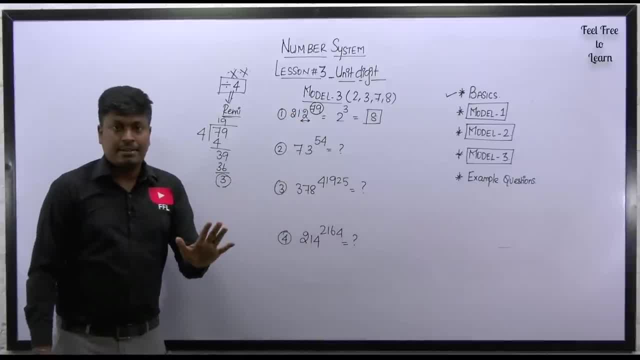 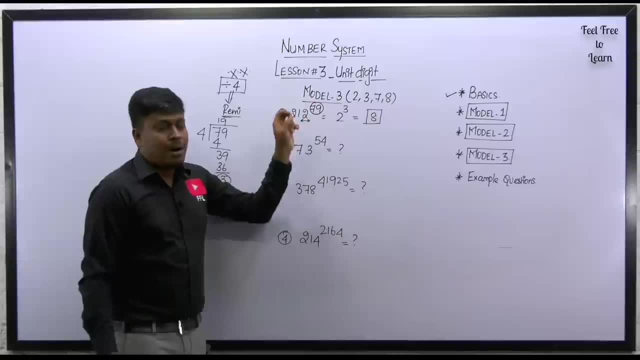 but after practicing this much of number you can able to understand it. But remember the logic first. what you need to do Is if you find the last digit of the given number is 2 or 3 or 7 or 8,. 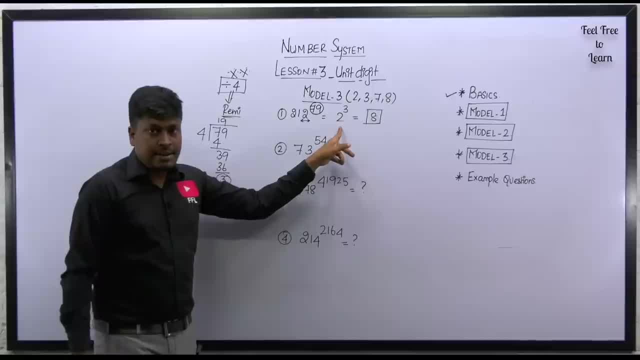 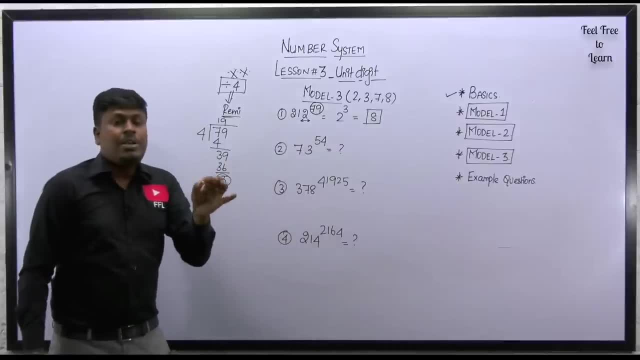 what you need to do is first write that number here and then you have to divide the power by 4, any power, So whatever the power they have given, you have to divide by 4 and you have to find the remainder. So, after finding the remainder, put the remainder to the power of the number, what you have written here. 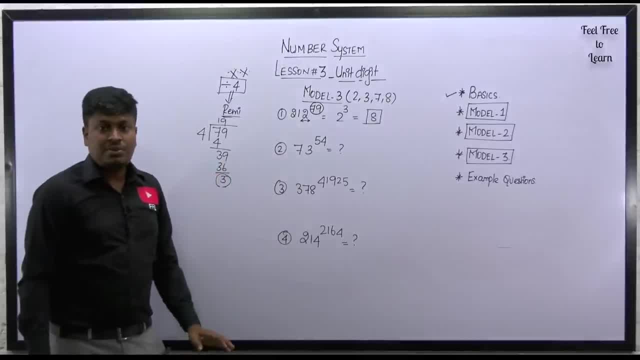 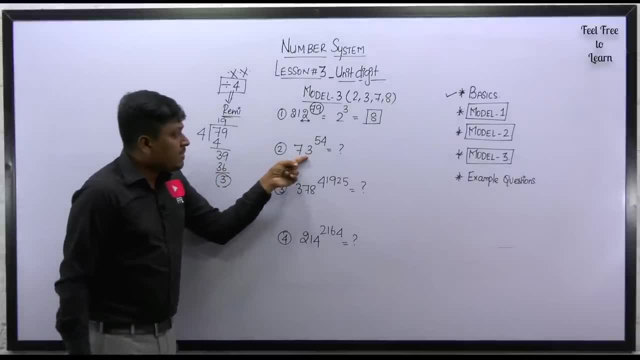 and then that will be the unit digit of your answer, understood or not. So let me take, let me move on to some other examples. You can able to understand it. So the second example is 73 power 54,. got it? 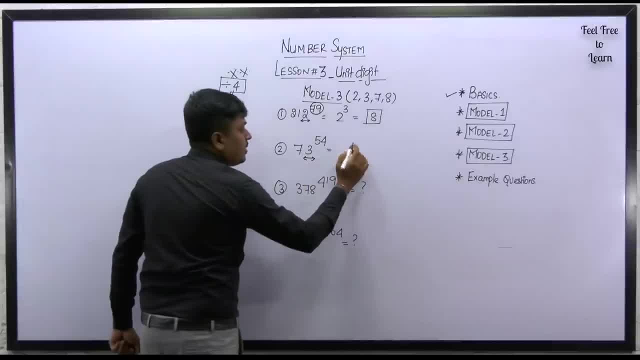 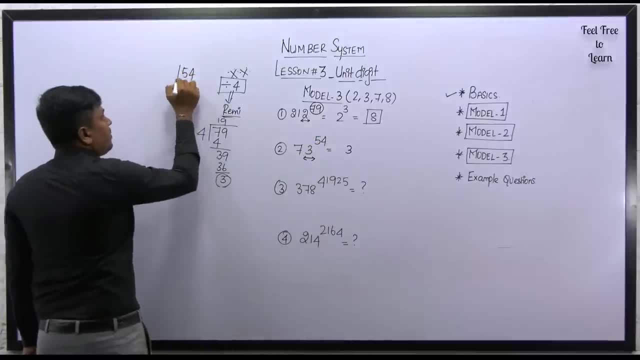 So here, what is the last digit? 3.. So first write down the 3 here, then what you have to do, You have to see the power. Power is what? 54. So divide this number 54 by 4.. 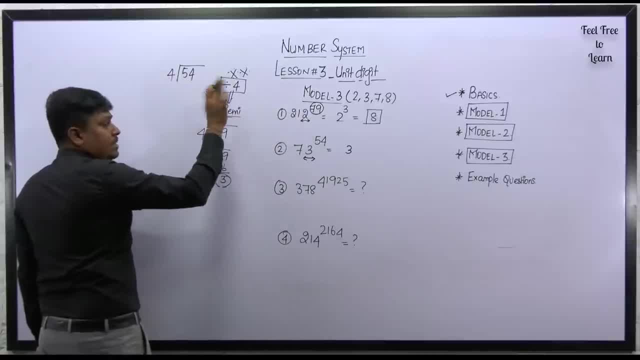 Always, whatever number be, you have to divide by 4.. That's the logic, right. If you divide by 4, 1, 4's are 4, so 14, 4- 3's are 12.. So reminder is what? 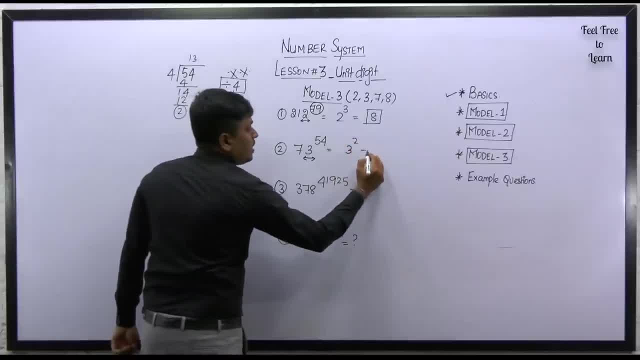 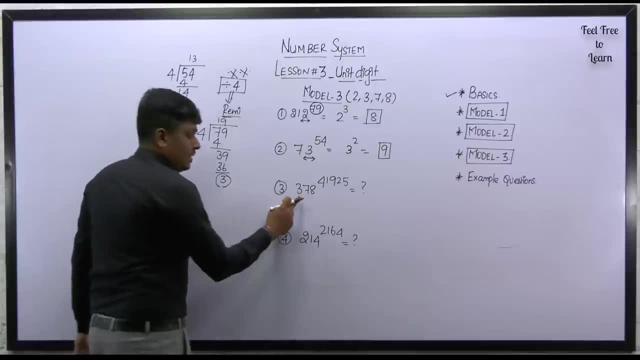 Reminder that we got is 2.. So write 2 here. 3 square is 9, that's it, got it. So unit digit will be 9.. Next question: 378, 41925, power 41925.. 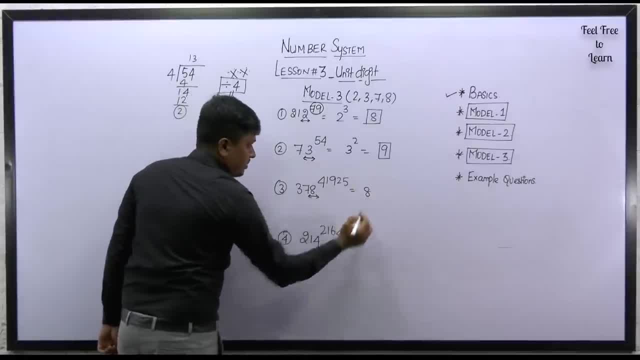 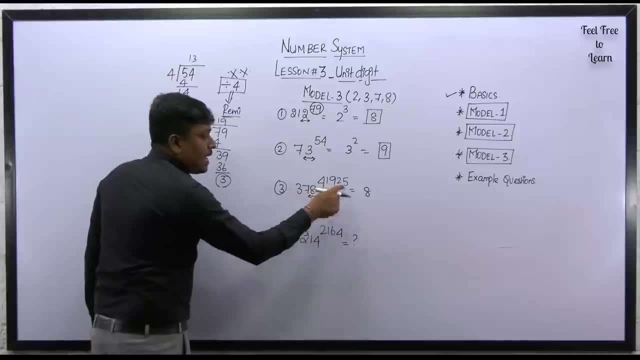 Last digit of the given number is what Write down: 8 here. another important thing: Just look at the numerator, just look at the power. right, So power is 41925.. You don't want to divide the complete 49215.. 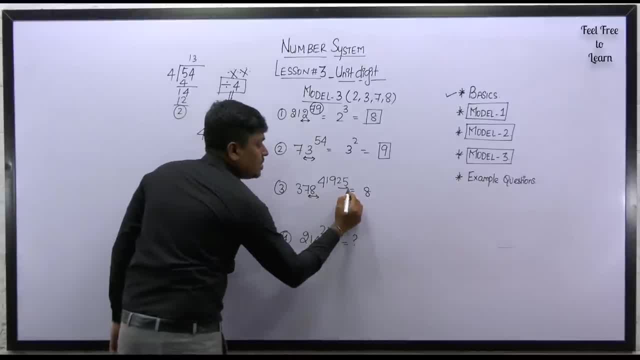 It's 41925.. It's waste of time. You just take only the last 2 digit of the number. What is the last 2 digit? It's 25.. Divide only the last 2 digit of the number by 4, right. 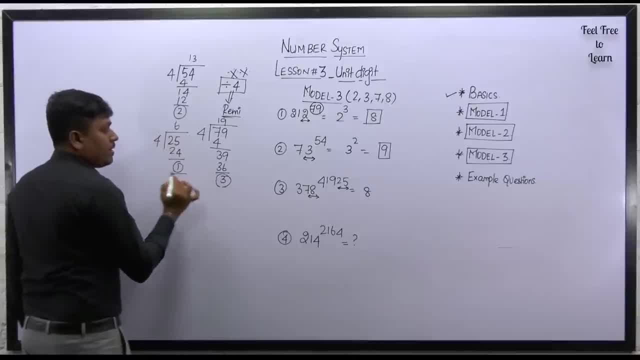 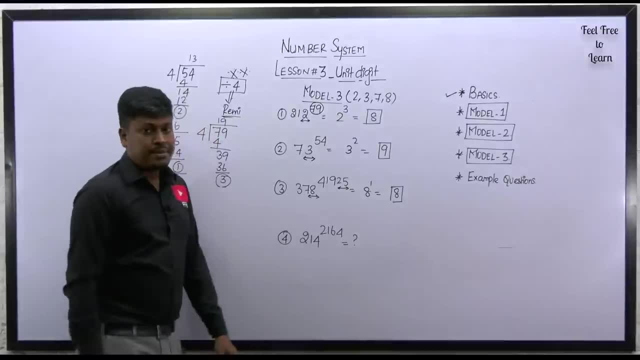 So 6, 4's are 24.. What about the remainder here? Reminder is 1.. So put the remainder here: 8 power 1 is 8.. So we can say that the unit digit will be 8.. So, friends, understood or not? 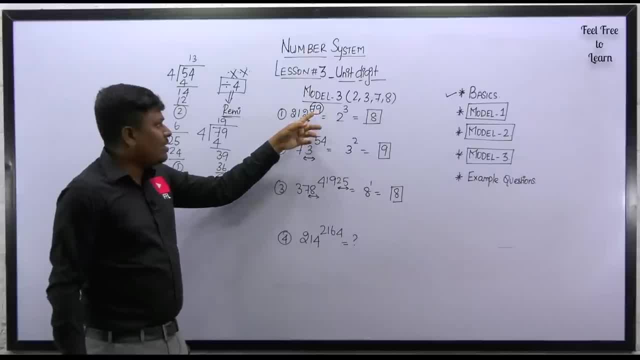 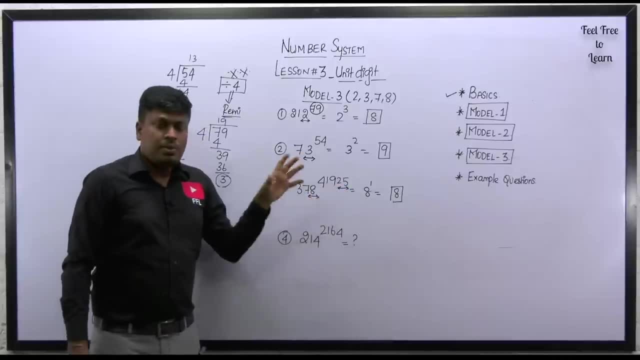 So already here I have, already we have 2, the powers, that we have 2 numbers, So 2 numbers. But here alone you can, You can able to see: the power is 41925.. You don't want to divide the complete, all the digits, by 4.. 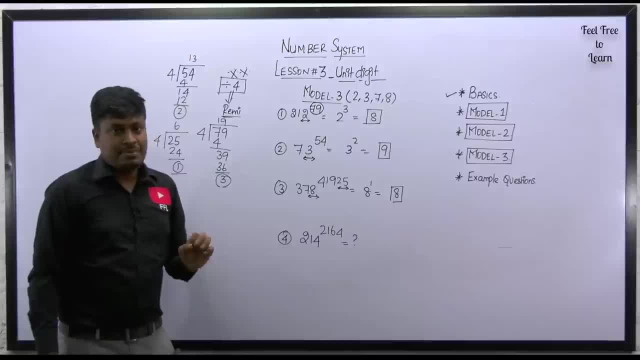 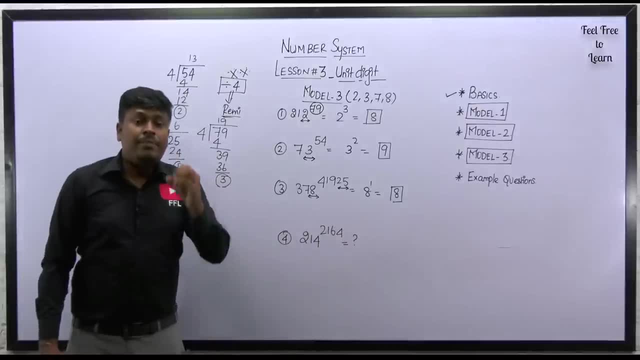 It is better to divide only the last 2 digit. That is enough, Got it. So finally, we got the remainder 1, write down the remainder here. So 8 power 1 will be 8.. In case, if we got a remainder 0, right. 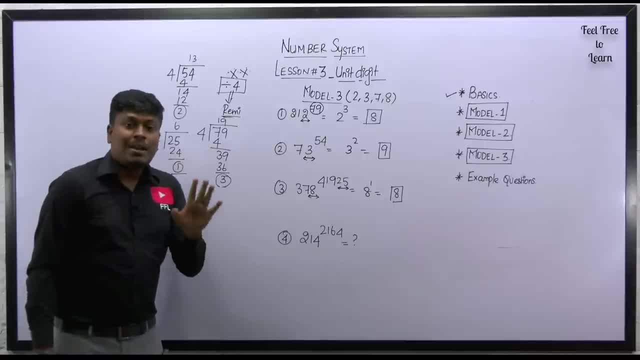 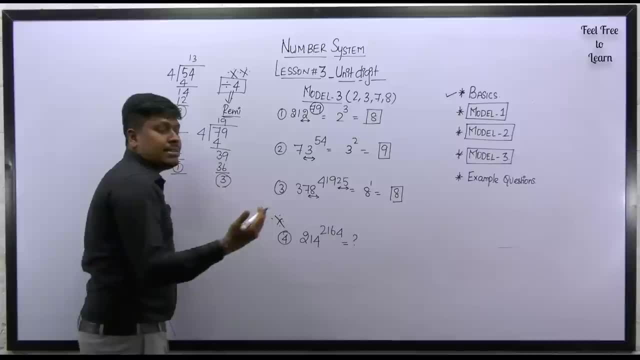 If we got a remainder 0, what you need to do is you need to write down 4 and then you have to find the unit digit. Just look at this last number. number 4 alone is an exceptional case If it gets a remainder 0.. 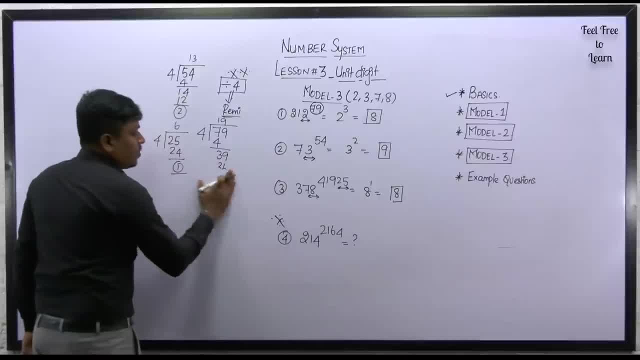 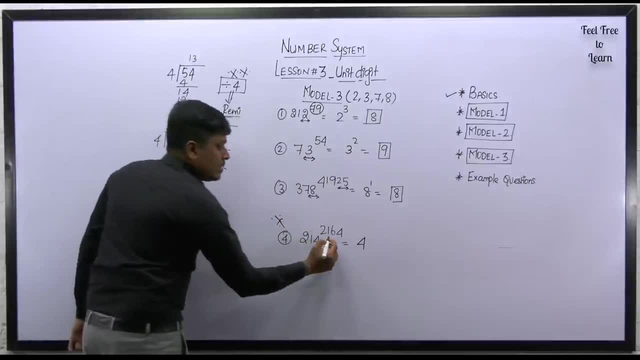 So 214 power 2164, right? So first what you need to do, the last digit is 4.. So write down 4 here and 2164.. You don't want to take all the 4 digits, Just take only the last 2 digit. 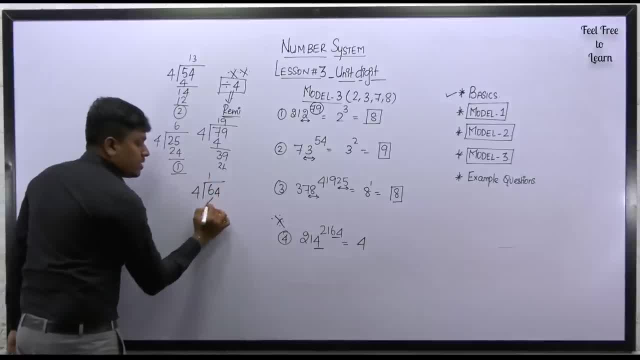 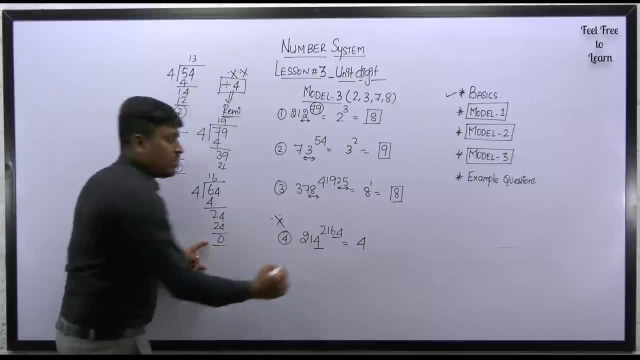 So 64 divide by 4.. So 1, 4's are 4.. So remaining will be 24.. 6, 4's are 24.. So what is the remainder that we got here? 0.. You should not write down 0 here. 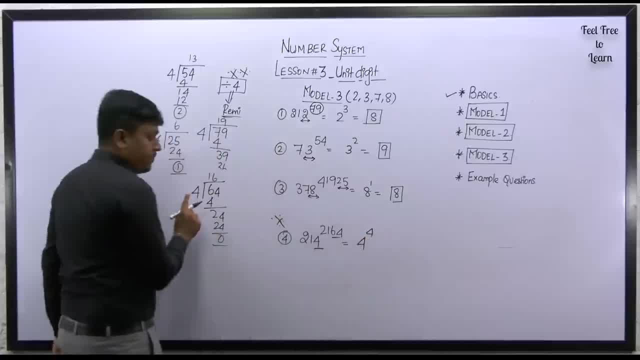 You should write 4.. You got it Because we are dividing by 4, right? If we get a remainder 1,, 2,, 3, etc. Put the numbers there. If you got a remainder 0, put number 4, because we are dividing by 4.. 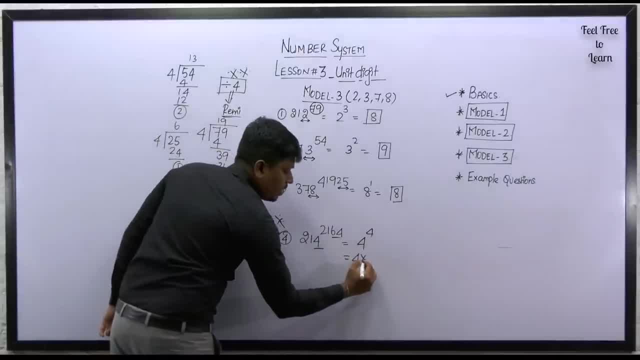 So put number 4 here, So 4 power 4.. So 4 into 4 into 4 into 4. for easy calculation: 4: 4's are 16, right 4: 4's are 16.. So 16 into 16.. 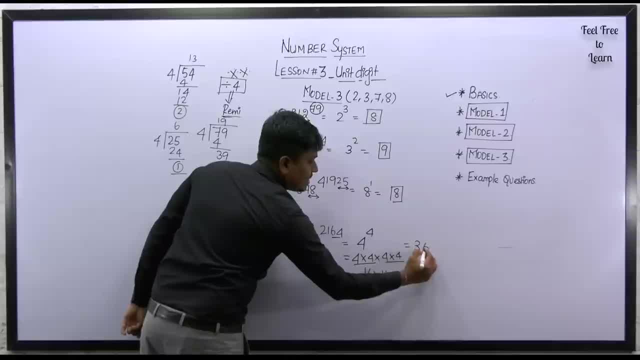 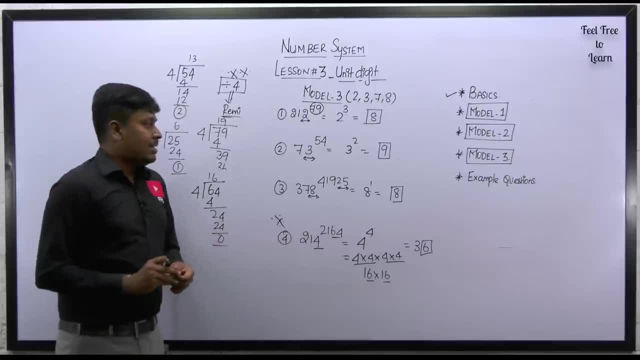 6 into 6 will be 36.. So 36,, the last digit will be 6.. So we can say that the unit digit will be 6.. So friends understood right. So in this model number 3 is little bit tricky, but it is easy if you understand the concept. 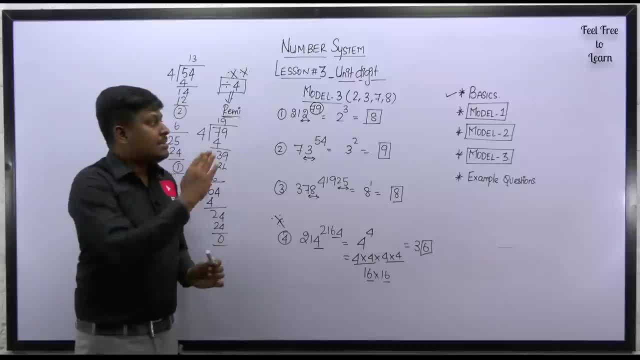 So what is the concept I have told you is if the number that ends at 2,, 3,, 7 or 8, first step, what you need to do: write down the numbers, right? If it ends at 2, write down here. 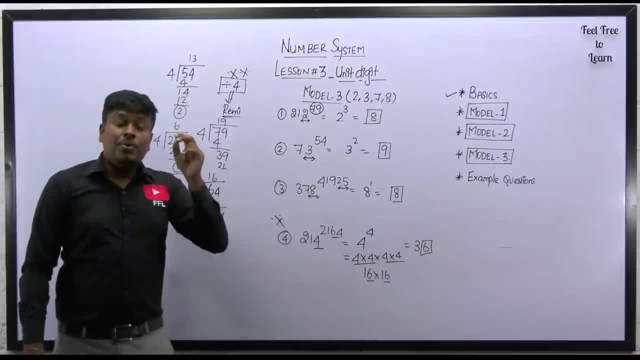 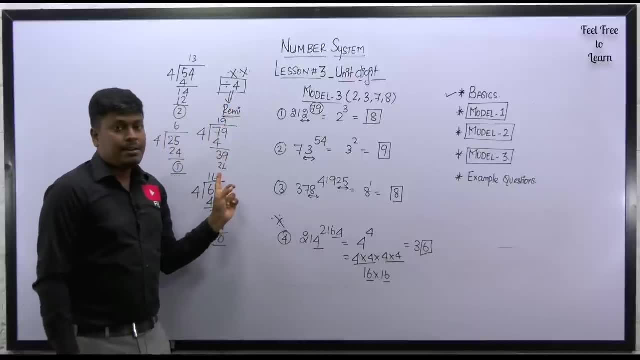 If it ends at 3, write down here. Second step: you need to look at the powers. Always, the power should be divided by 4, right After dividing, find what is the remainder. If you got remainder 1,, 2,, 3,, 4, whatever remainder, we put it in the numerator of the number. what you wrote here already. 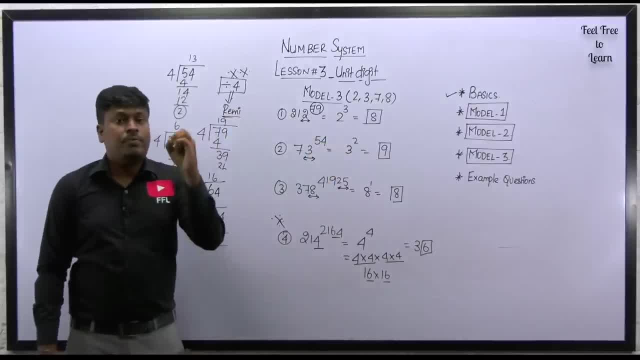 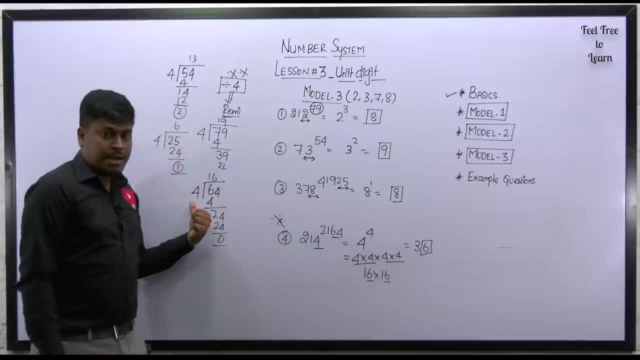 So and then find the unit digit, In case, if you find the remainder 0,, if you got the remainder as 0, you have to use 4 power 4.. So you have divided by 4, right, So write down the 4 here, because you should not write 0 here. 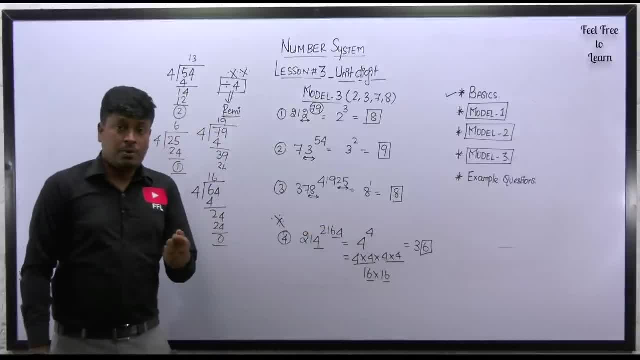 So write down 4 and then find the answer. Another important note is: don't divide, always don't divide the complete, all the numbers. It is better to take only the last two digit number and divide by 4. You will get the answer. got it. 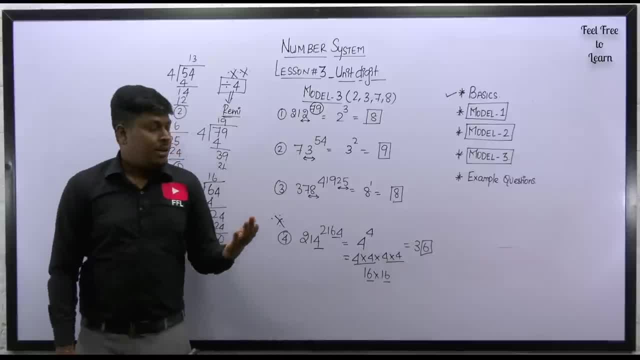 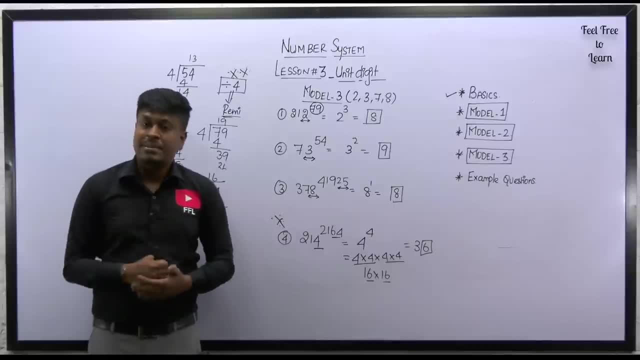 So now, after learning this, model number 1,, 2,, 3 and 4, now let me move on to some example question that was asked in previous competitive exams, so that you can able to understand the concepts completely. So, finally, we can go with some example questions here. 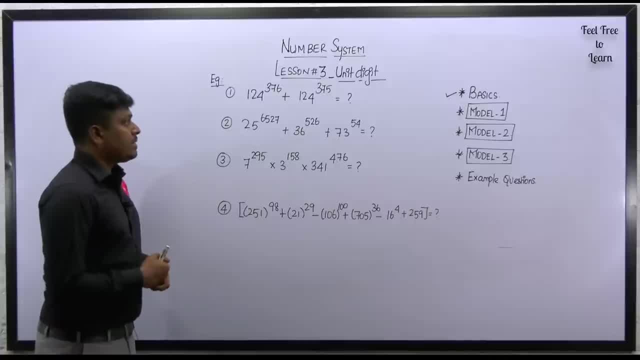 So first question: 124 power 376 plus 124 power 375.. So when just see here always if we need to find the unit digit of these numbers. so every time while solving a number, check which number it is, which model it is. 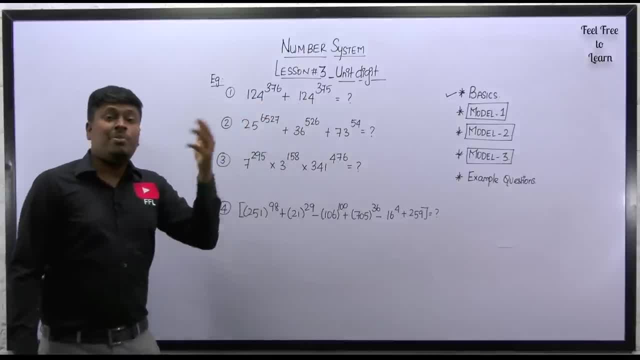 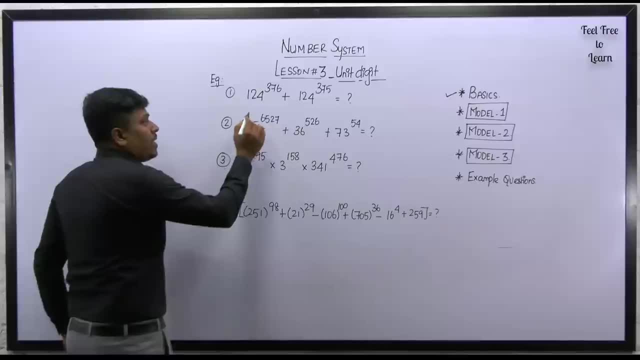 So number 4 here, model number 2, number 2. if it is model number 3, number 5, it is model number 1.. So that it is easy to solve the question, got it. So first question 124, power 376.. 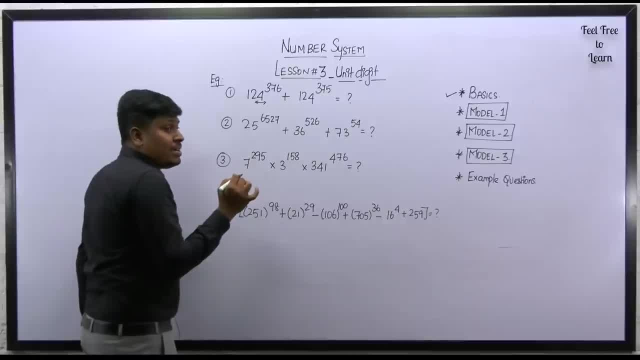 So the last digit is 4 here. So 4, in which model we have learnt Model 2.. So 4 power 376,. 4 power, even number. If it is 4 power all, it is odd, it is 4.. 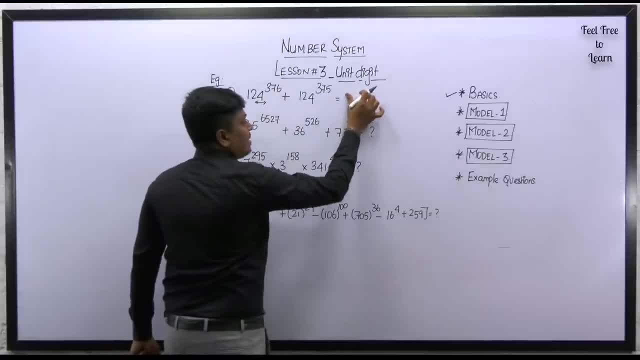 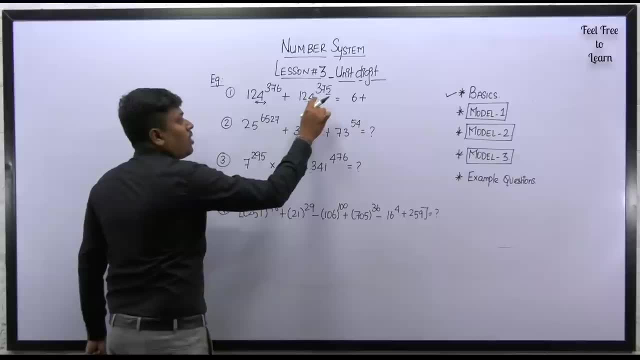 4 power even will be 6.. So 4 power even. so we can say that the unit digit will be 6.. So 4 power odd. here 375 is odd, So 4 power odd will be 4.. So 6 plus 4 will be 10.. 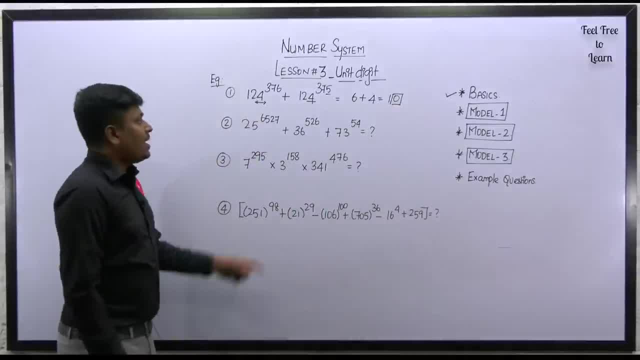 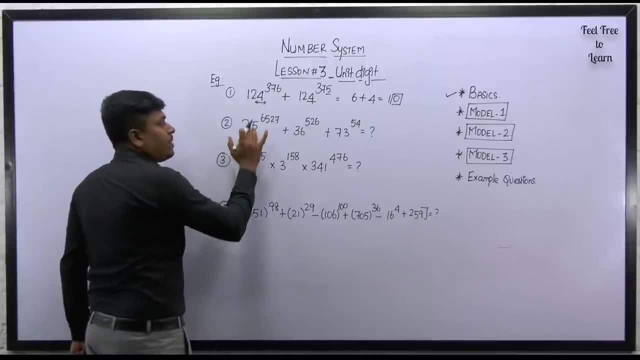 So finally we can say that the unit digit is 0.. So answer for first equation where the unit digit is 0.. Friends understood. So question number 2, see 25 power 627,, 36 power 526,, 73, power 54. 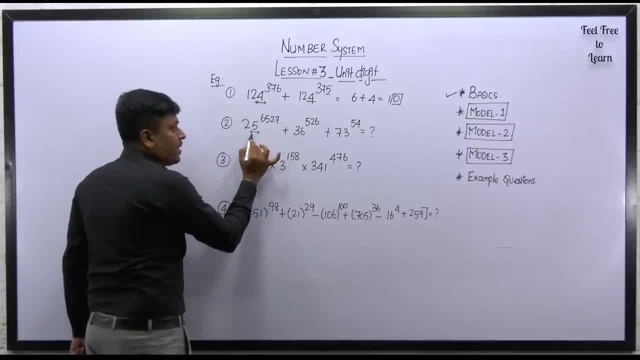 So first look at the last digit of the number is 5.. So number 5, we have learnt in which model Model number 1. 5 power, anything is 5, right. So 5 power, 6527, not to worry about it. 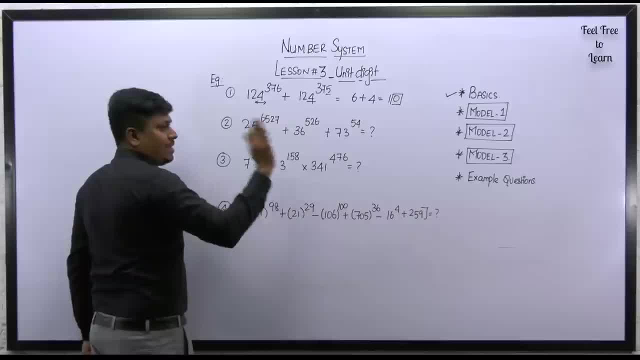 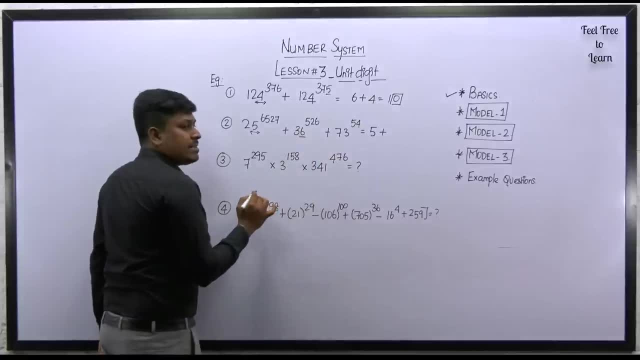 By seeing a number. do not decide, it is difficult. So 5 power, anything is 5.. So we can say the unit digit is 5.. So plus 6.. Again, model number 1, we have learnt this number 6.. 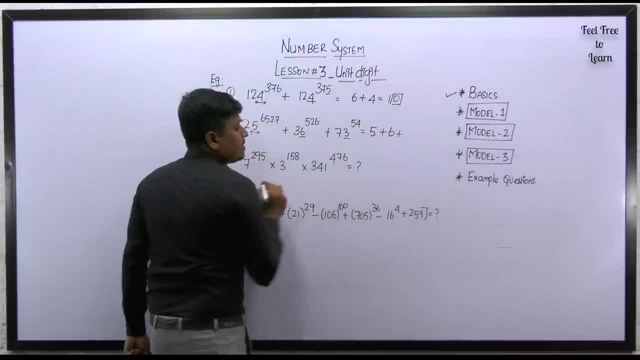 6 power. anything is again 6.. Plus last is 3.. So 3, we have learnt in the third model, So third model alone. we have to divide the power by 4.. So write down 3 here. What is the power here? 54.. 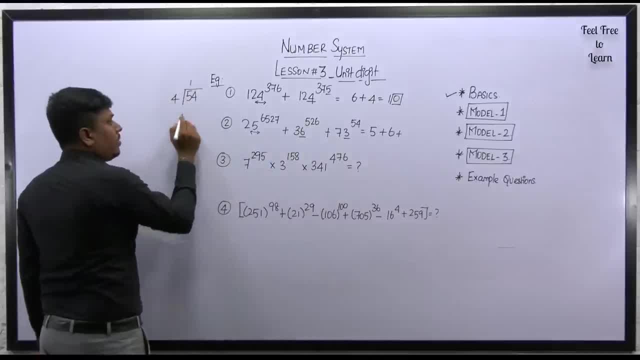 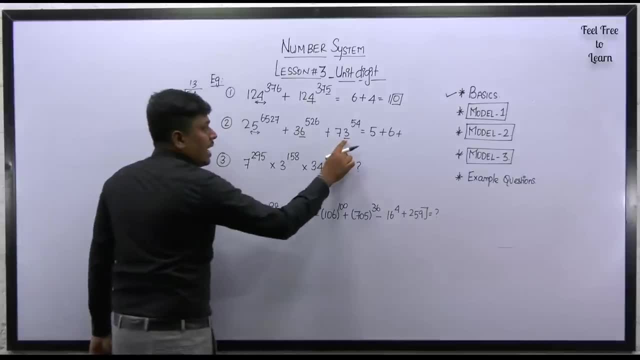 So divide 54 by 4.. So 1, 4's are 4.. So remaining will be 1, 14.. 4, 3's are 12.. So what about the remainder? here is 2.. And here we have number 3.. 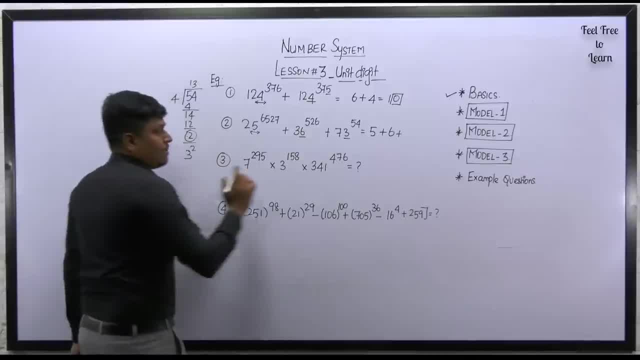 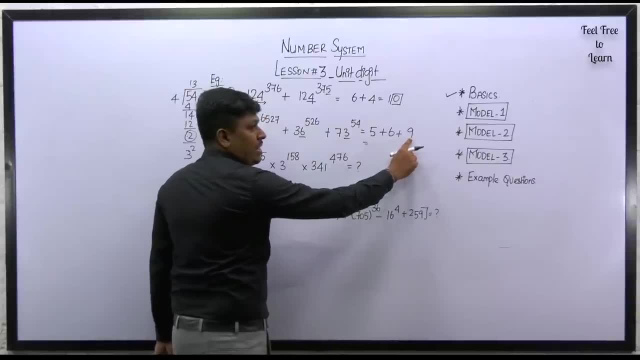 So write down 3 here. Reminder is 2.. 3 square will be 9.. So write down 9 here. got it. So now we need to add it. 6 plus 5 will be 11.. 11 plus 9 will be 20.. 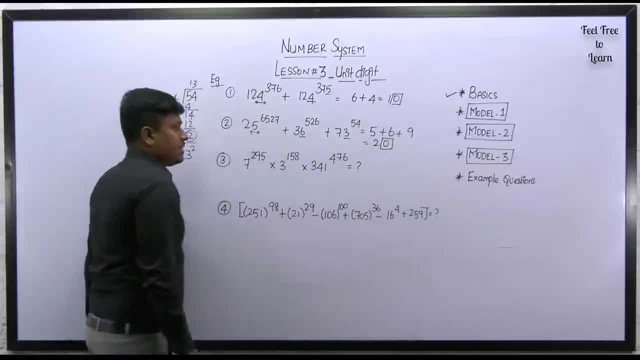 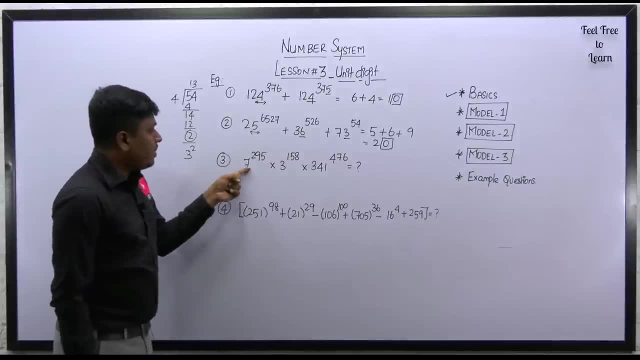 So 20,. the last digit is 0.. So finally we can say that unit digit of this number will be 0.. Understood, So question number 3.. 7 power 295,. 3 power 158, 341 power 476.. 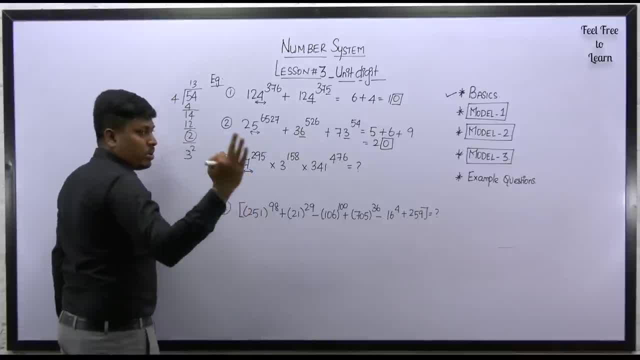 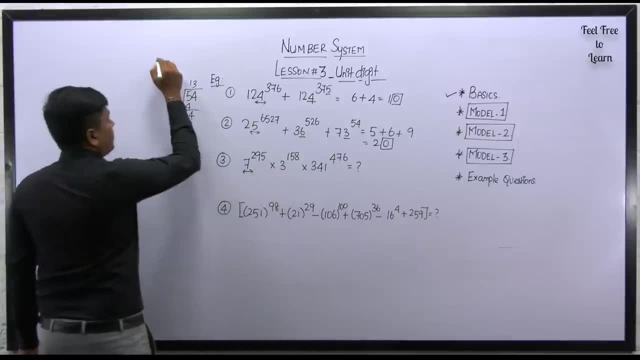 So here, 7.. 7, in which model we have learnt, Model number 3.. So model number 3, we have to divide the power by 4.. Got it, Just take only the last 2 digit, That is 95.. 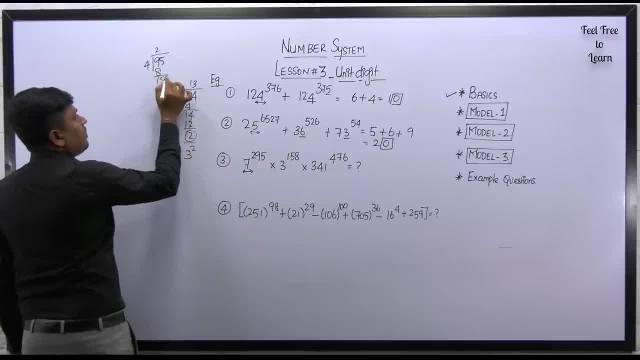 So 95 by 4, 4: 2's are 8. Reminding 15. So 4: 3's are 12. Reminder will be 3.. So got it. So 7 power, remainder 3. That is, 7 power 3 will be 343.. 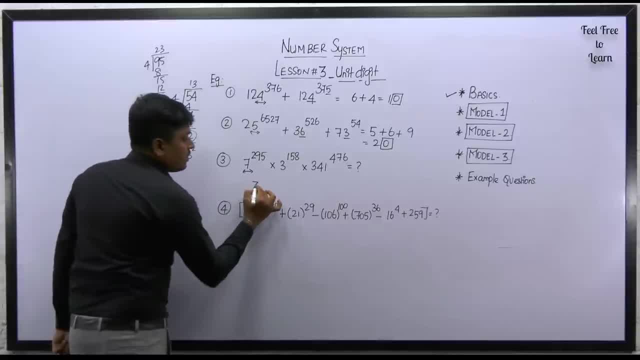 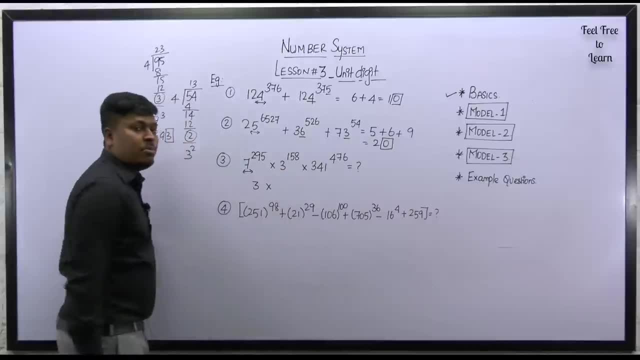 So we can say that the last digit will be 3.. So unit digit of the number is 3.. Got it So into? so 3 power 158.. Again, this 3 we have learnt in model number 3.. What you need to do: 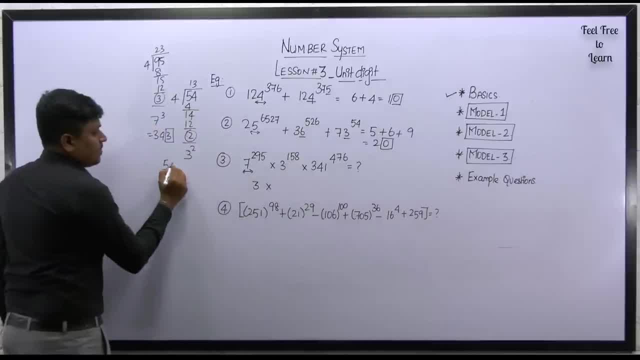 Similar process. Take the last 2 digit, That is 58 divide by 4.. So 1: 4's are 4, 18.. 4- 4's are 16.. Reminding will be 2.. So reminder is 2.. 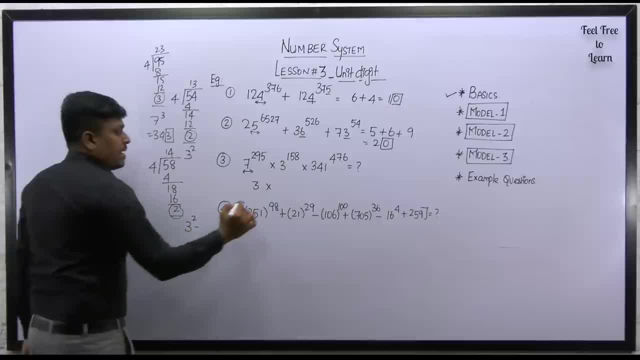 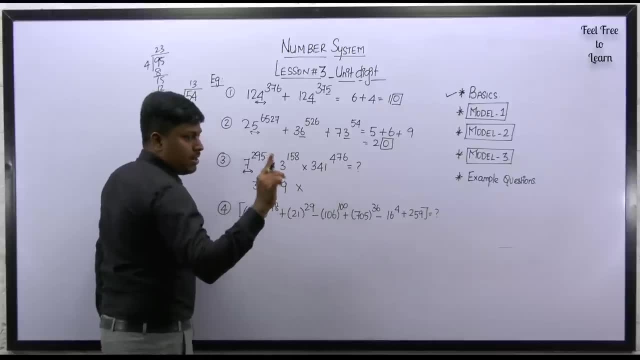 Already we have number 3.. So 3 power 2 will be 9.. So we can write down 9 here Into. so the last digit is 1.. So 1 we have learnt in model number 1.. 1 power anything is 1.. 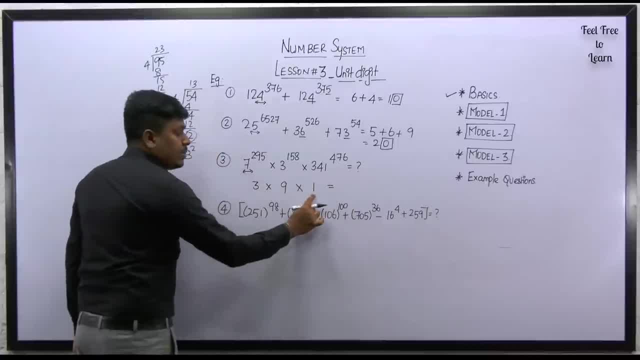 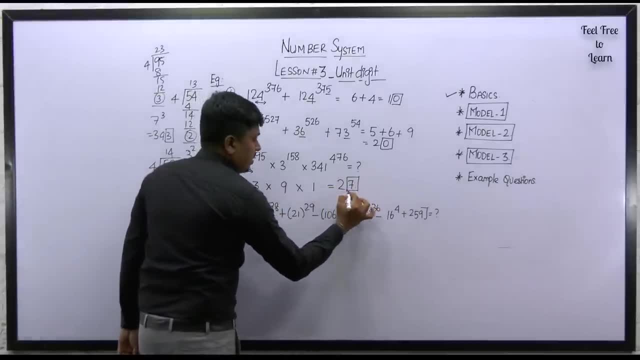 So we can say unit digit is 1.. So 3 into 9 into 1.. 9 into 3 will be 27.. 27 into 1 will be 27.. So the last digit will be 7.. So finally we can say that unit digit of question number 3 is 7.. 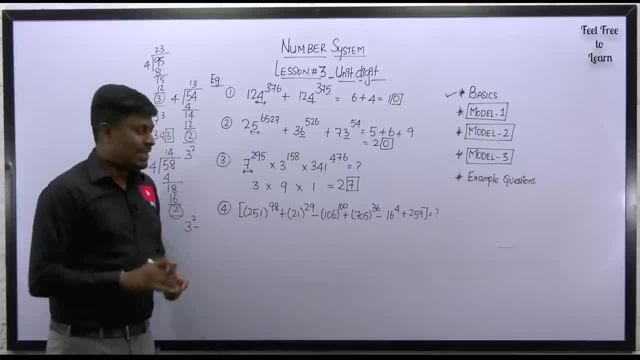 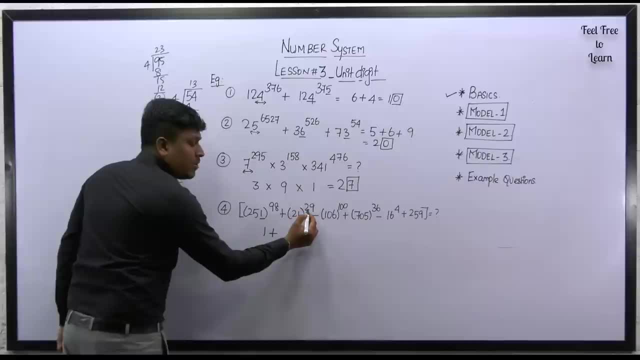 So last question. See, the question looks lengthy, but solving is easy. Just see here: 1 power 98.. 1 power, anything is what 1.. So plus again, 1 power 29.. 1 power, anything is what. 1 minus of 6 power 100.. 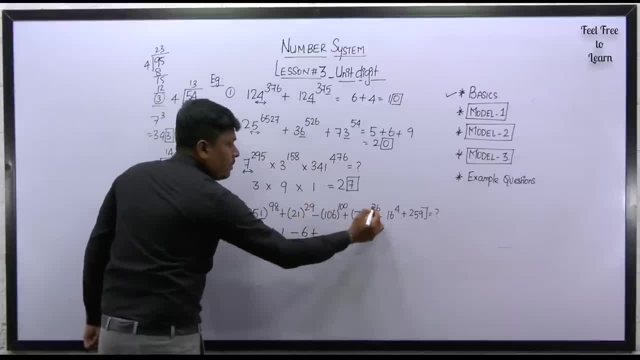 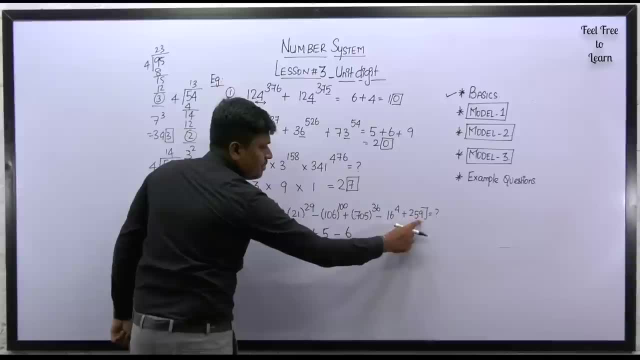 6 power, any number will be 6.. So plus 5 power, any number will be 5.. Minus of again 6 power, any number will be 6.. So the 259 power is nothing. So we can say the last digit will be 9.. 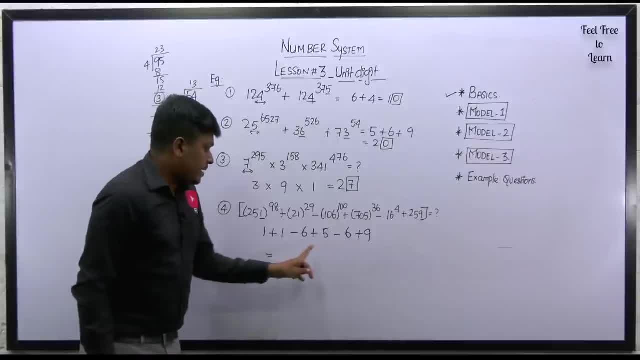 So add all the numbers here So we can add 9 right. 9 plus 5 will be 14,, 15 and 16.. So total is 16 minus of minus 6. minus 6 will be minus 12.. So finally we can say that 16 minus 12 will be 4.. 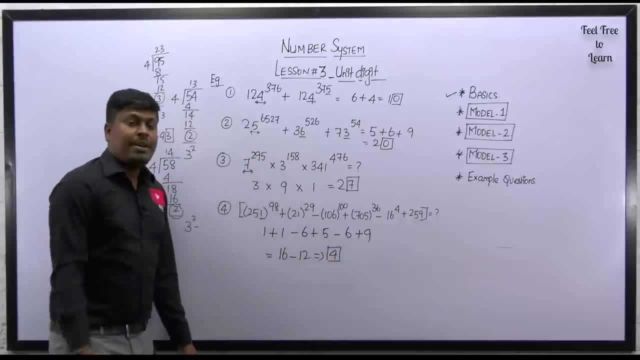 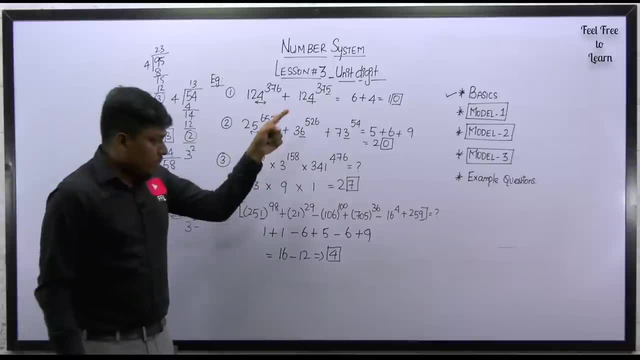 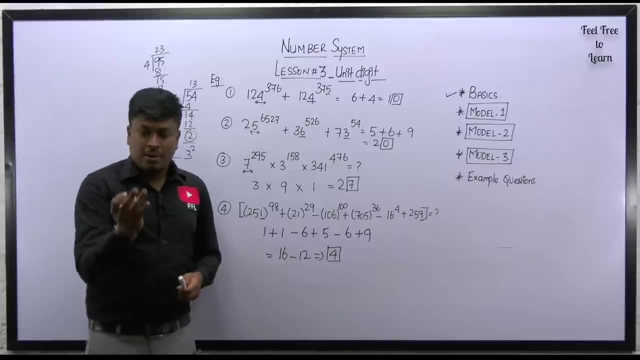 So which is the unit digit of the number? So finally we got unit digit, that is 4.. So once finally we have solved 4 example question. So all these 4 questions were previously asked in many competitive exams. See, if you learn that model number 1, model number 2, model number 3,. 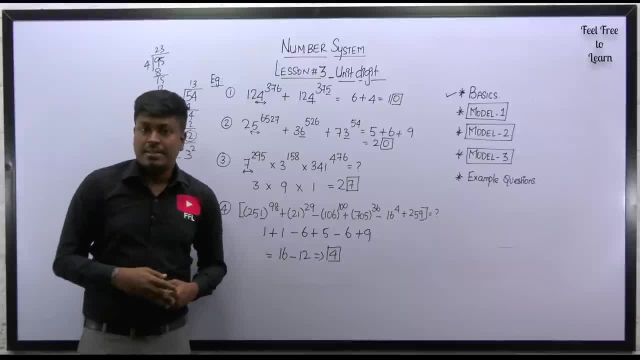 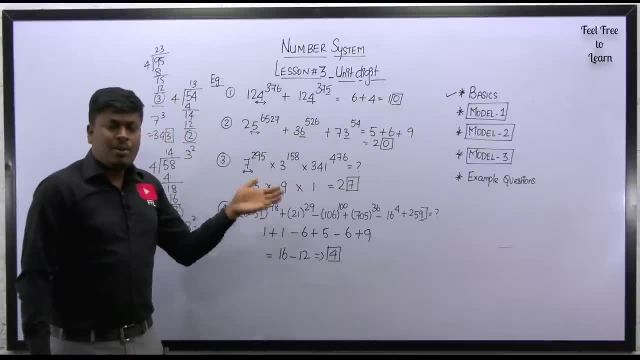 you can able to solve any question on this unit digit, But it requires some practice. This question is not enough. Just take your books. if you have any railway books, or a search in Google Find unit digit, You can able to find many questions. 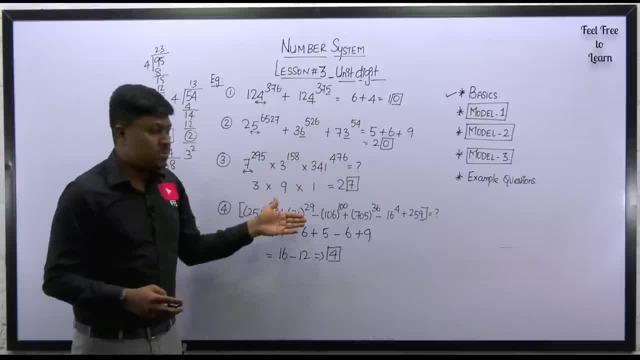 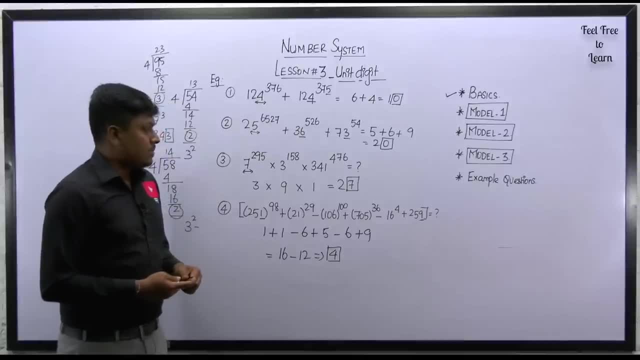 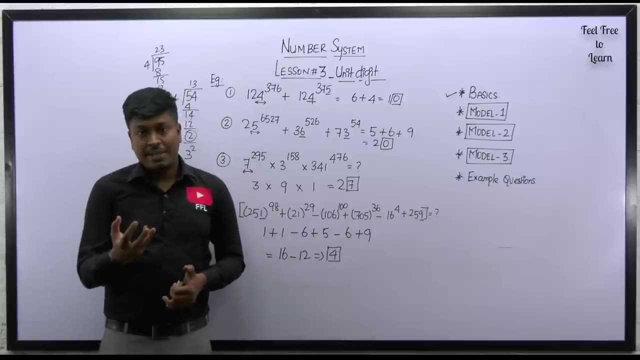 All the questions. try to apply this model and try to solve it, Surely you will get the answer. So once got it, So that's it about this unit digit. So next lesson we can learn new, new concepts on this number system topic, because number system is the basics of quantitative aptitude, right? 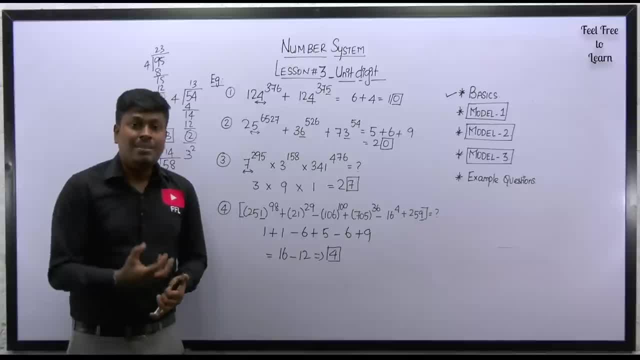 So that's the reason we are taking more number of time and more concepts to teach this number system. So once that's it about unit digit. Thank you so much for watching this video. If you really like it, share the video to your friends. 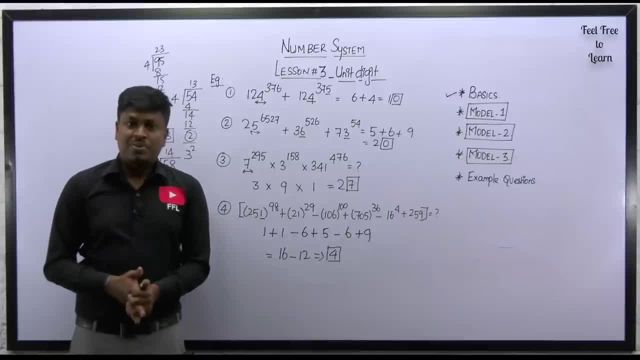 Those who are preparing for the competitive exams. So thank you so much for watching it. Bye. 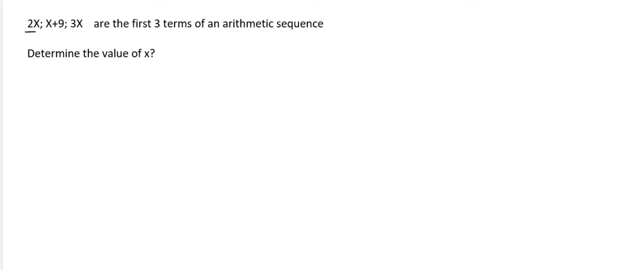 Hello everyone. so in this sequence we are given three terms and they tell us that these are the first three terms of an arithmetic sequence determine the value of x. So the way you approach a question like this is the following: We know that in an arithmetic sequence the difference 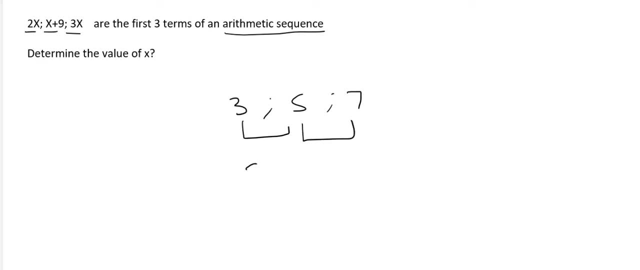 between the numbers stays the same, So we could say that 5 minus 3 will always be the same as 7 minus 5, and if we had to carry on, then that would be 9 and you could say that that must be the same. 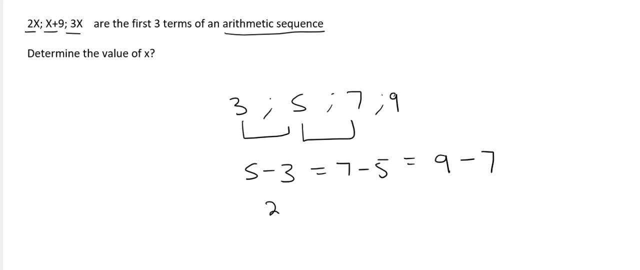 as 9 minus 7, because 5 minus 3 is 2,, 7 minus 5 is 2,, 9 minus 7 is 2.. So you could say something like t3 minus t2 is always the same as t2 minus t1. or you could say: t10 minus t9 is the same as. 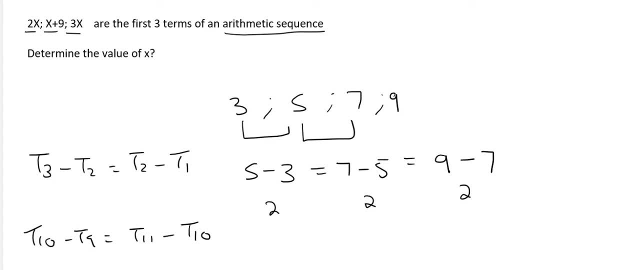 t11 minus t10 or whatever you like, as long as you always say a term on the right minus a term to the left. So a term on the right minus a term to the left, a term on the right minus a term to the left.